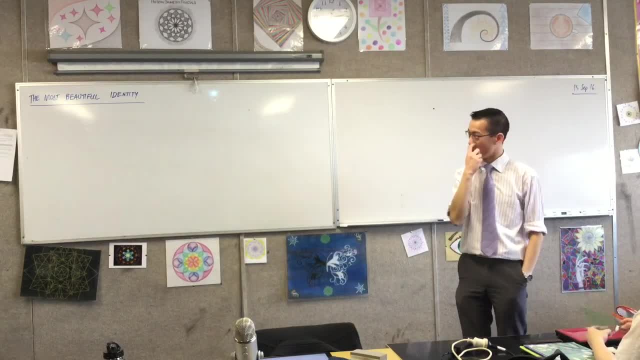 pieces, And I kind of think, because I know a lot of you- for a significant number of you, despite the fact that this is the class it is, a significant number of you will never do maths again after this class is over, At least in a formal sense, And so I view it. 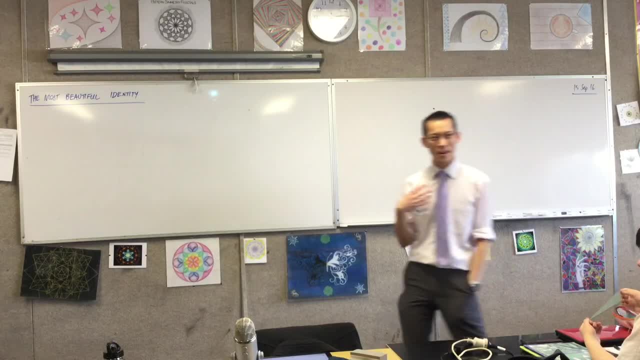 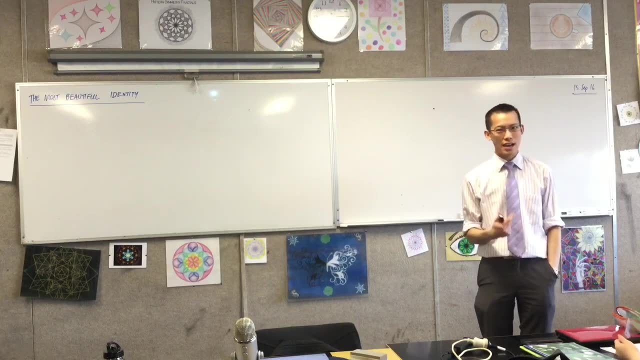 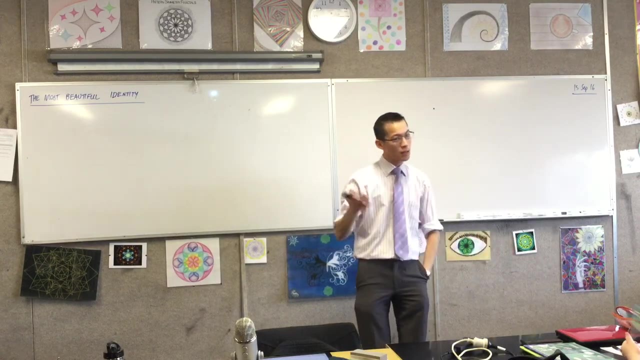 as an immense tragedy that you never get to meet this. But it takes some work to get there, which is why you're not supposed to know it, because it's outside the scope of the course. It's outside the scope of any interesting course, in fact. So it's built upon an idea. 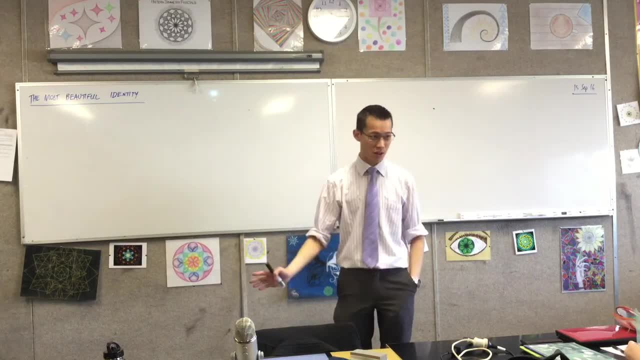 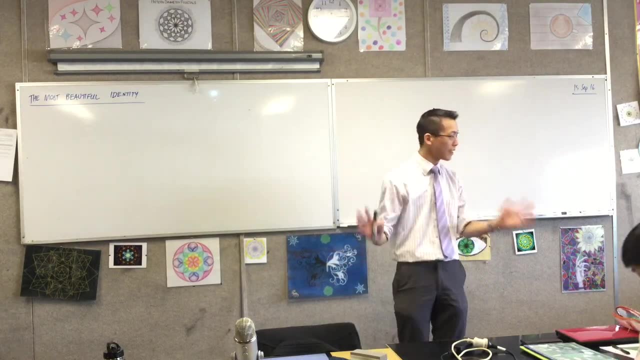 that we sort of meet in Extension 2, but I want all of you to know it. So this lesson kind of has three acts. The first act is we're going to look at in very, very just the bare details which everyone can get of the idea in Extension 2, which 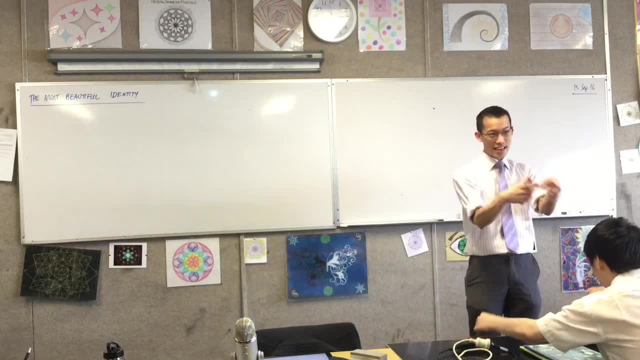 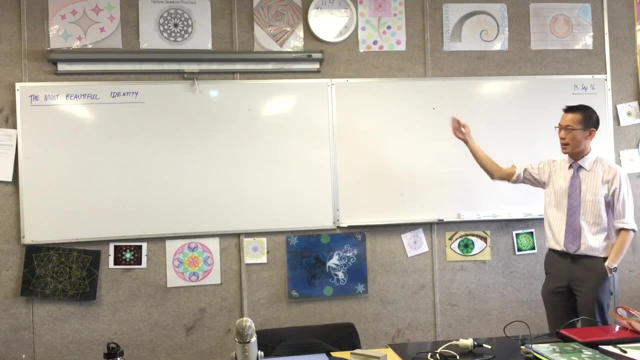 is built on. Then we're going to build a second idea which is not even in Extension 2, so that'll be new ground for everyone. And then the third act is. I'm going to show you what this idea is Now. I should also point out this is often called the most beautiful formula. 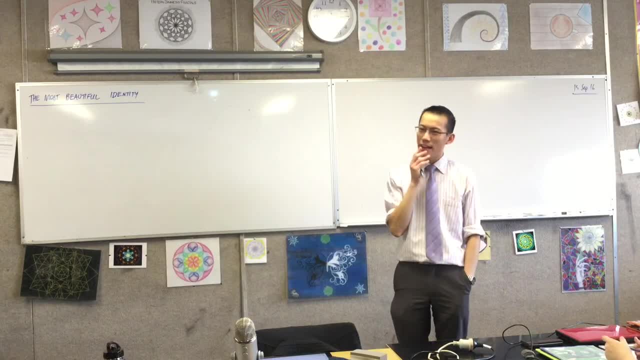 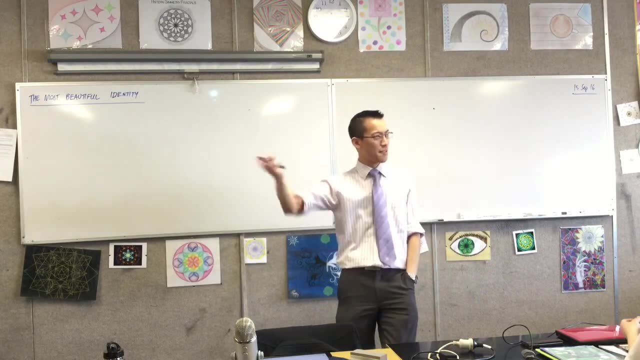 This is one of the reasons why I'm so keen to show it to you All of the like, because this is what mathematics is. you know how, like on, like BuzzFeed, there's like top ten, top ten fight scenes in Marvel movies or top ten, you know chicken. 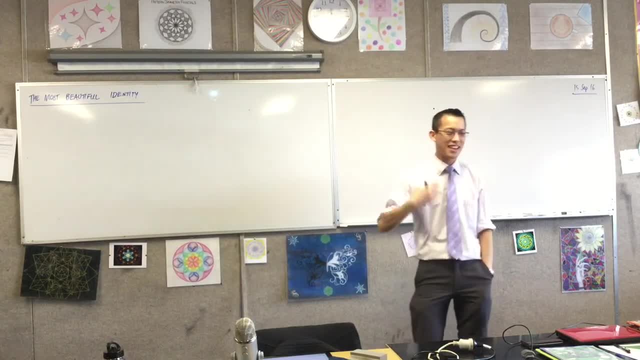 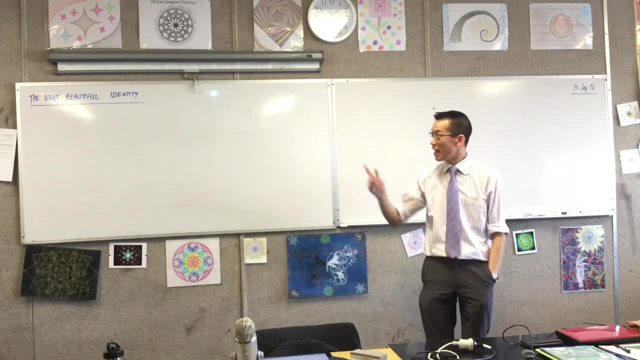 or whatever right. So people, people, always, there's this like innate human desire to come up with like top ten lists. right Now, on top ten lists for mathematical formulas, this one, without exception, universally, is always at the top every time. But I kind 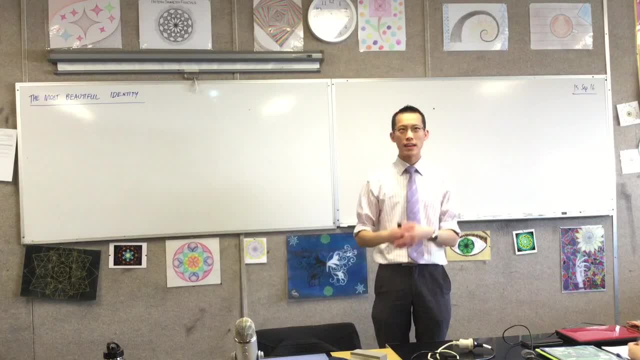 of think the word formula is a bit of a misnomer. When I think of formula, it's kind of like here's a set of steps you do to get something out the other end, right. Like there's a formula for the area of a circle, right It's. 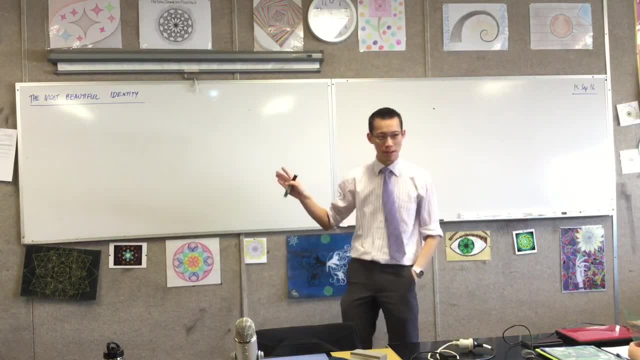 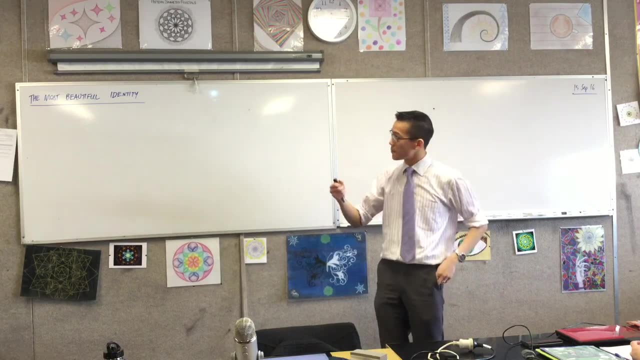 like: well, if you put this in, you get this out. okay, This is not a formula, it's an identity, It's a relationship between things that form two sides of an equation. okay, So if you haven't already make this heading and then just get ready to engage your mind. 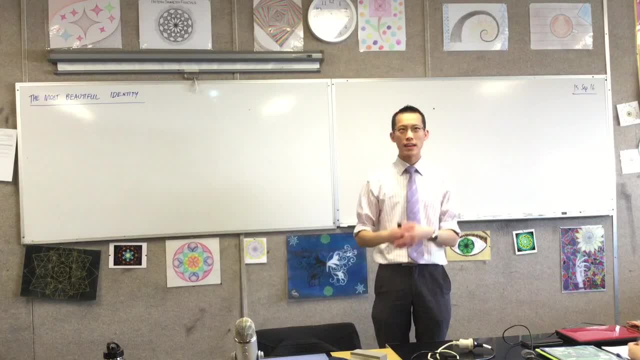 of think the word formula is a bit of a misnomer. When I think of formula, it's kind of like here's a set of steps you do to get something out the other end, right. Like there's a formula for the area of a circle, right It's. 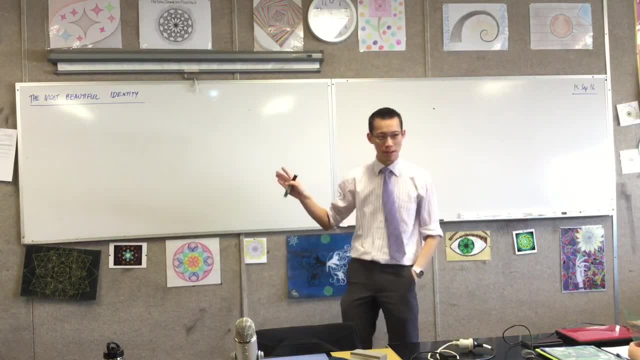 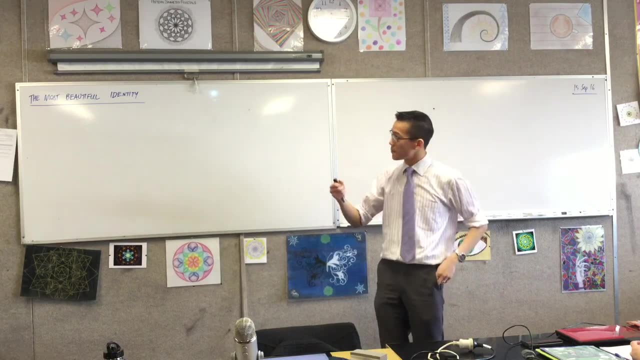 like: well, if you put this in, you get this out. okay, This is not a formula, it's an identity, It's a relationship between things that form two sides of an equation. okay, So if you haven't already make this heading and then just get ready to engage your mind. 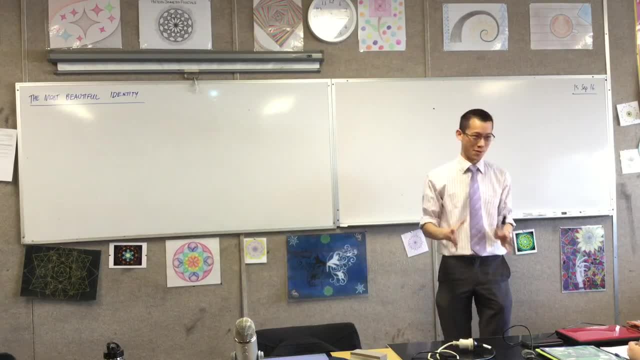 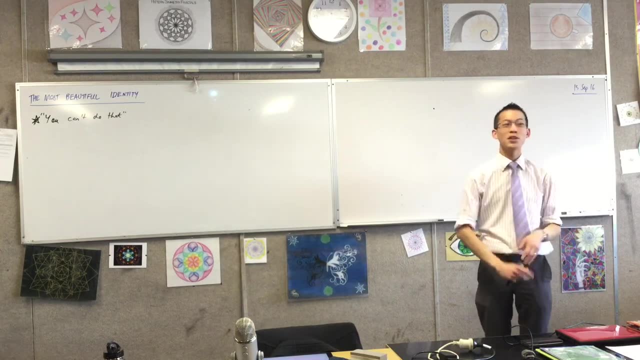 okay, Because we're going to go to some difficult places, but I promise it will be worth it, okay? Everyone in this room, regardless of how much maths I've been doing for the last two years, to understand this. okay, So I'm going to go right back to the beginning, okay, All? 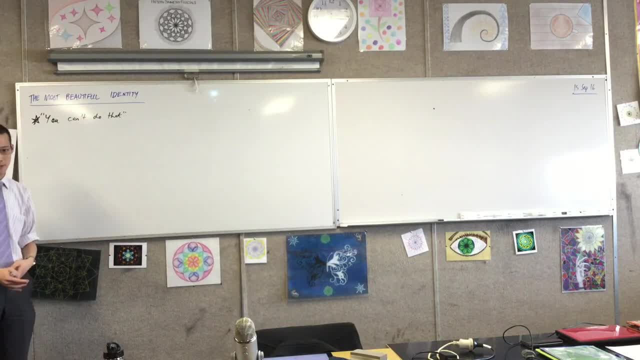 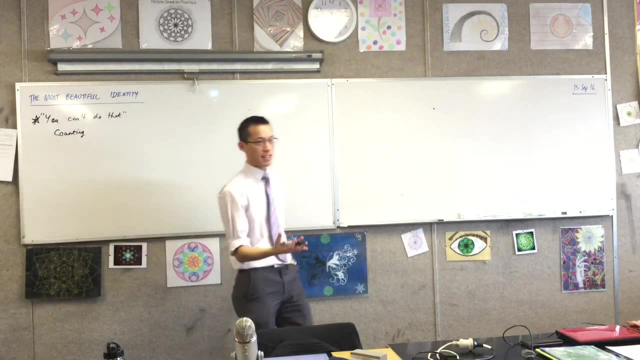 mathematics. in every culture throughout history, no matter where you are geographically, it always starts with the same idea, which is counting right, Even very, very young children have this concept of counting, so it's fairly sort of fundamental to the way we work and 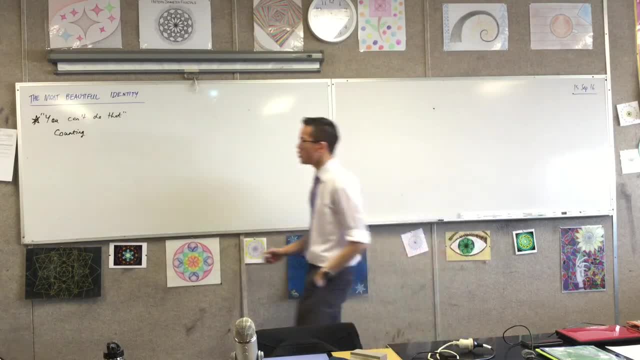 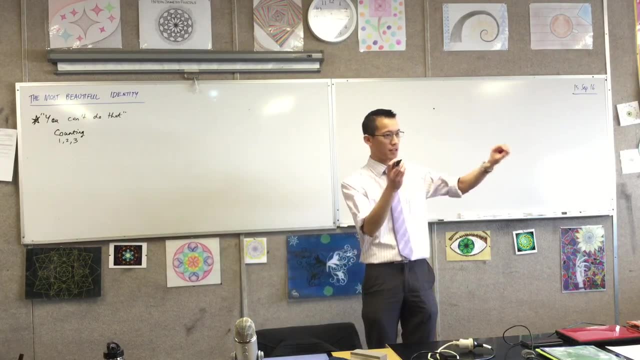 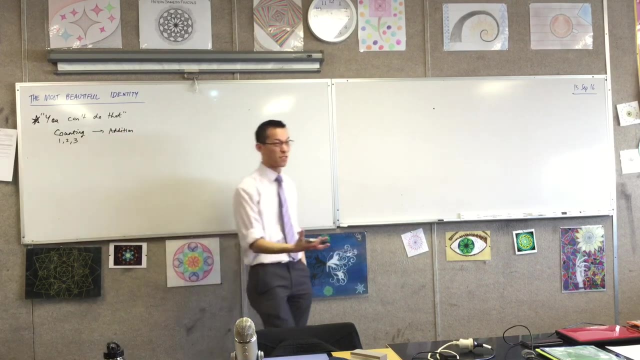 the way we sort of understand and interpret the reality around us. okay, So you start with counting, but as soon as you develop counting, It's fairly intuitive to move on from there to addition right, Like addition is actually. it begins just kind of as an extension of counting. right, You're plus 1, plus 1, plus. 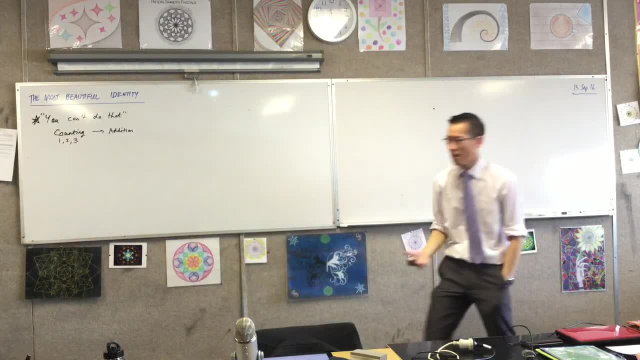 1,. and then you're like: well, why can't I add bigger numbers than that, right? So we can write something like: oh, I don't know, 11 plus 6 equals 17.. So addition comes out. 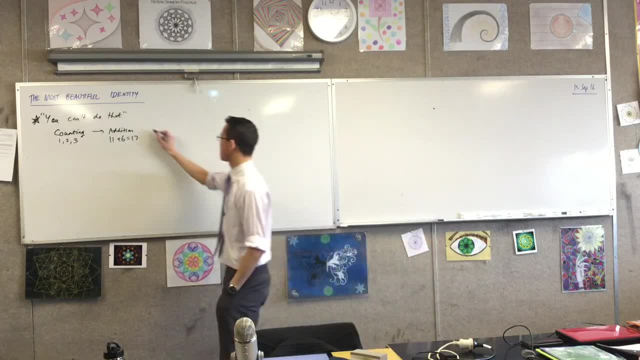 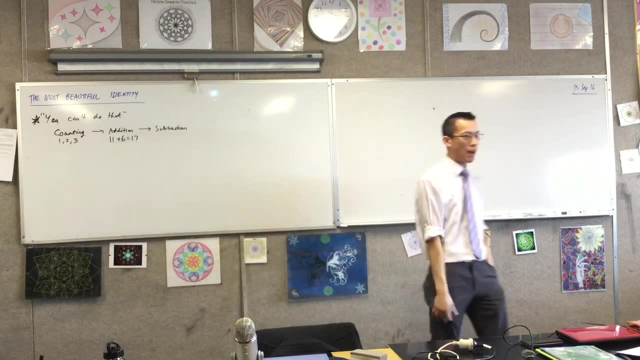 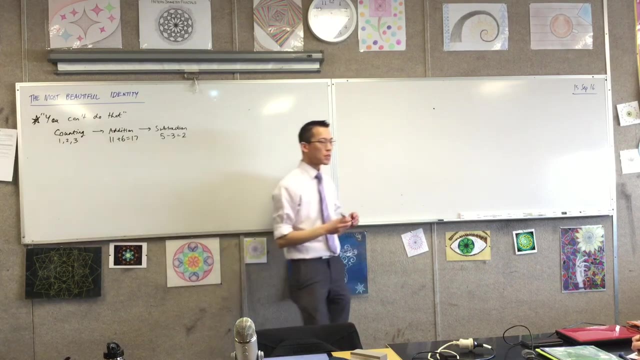 naturally. and then, as soon as you have addition, you have subtraction right, So you can put things onto a pile and you can take them away, and that's what subtraction is right. So we can write something like: 5, take away 3 equals 2.. Now, despite how little, 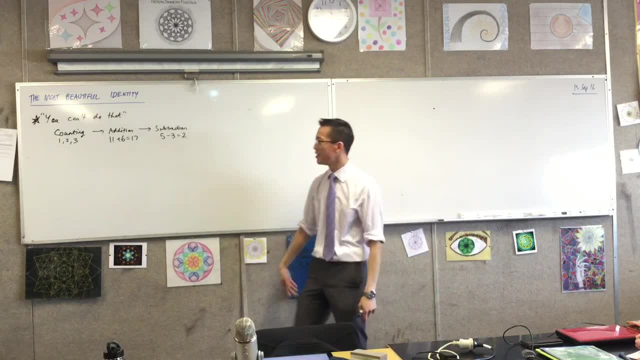 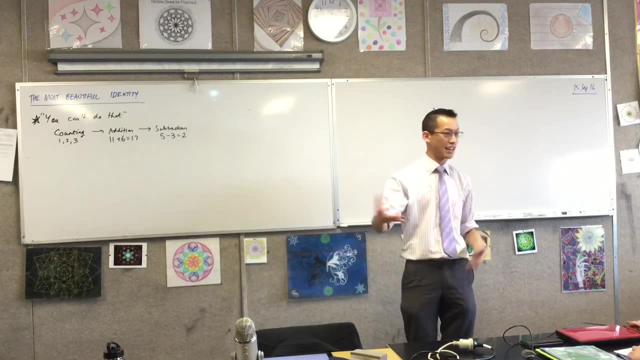 of a distance we have gone in terms of like mathematical concepts. okay, Counting and addition are incredibly free things. There are no rules really for counting an issue. You can count anything you like. In fact, that's one of the most amazing things about. 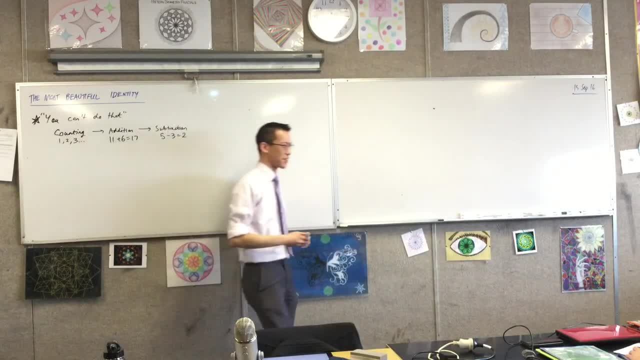 counting that. you know little kids. when they're like what's the biggest number you can think of? And they're like oh, 100. And you're like it's 101. And they're like oh. 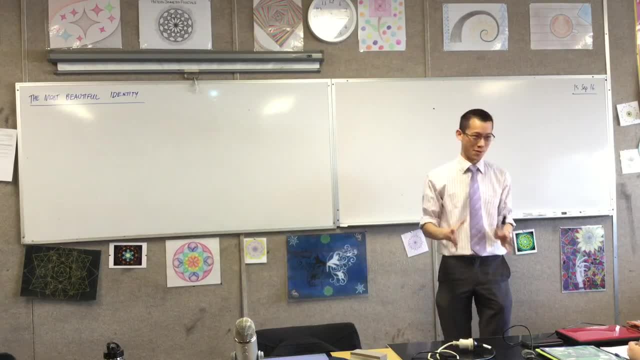 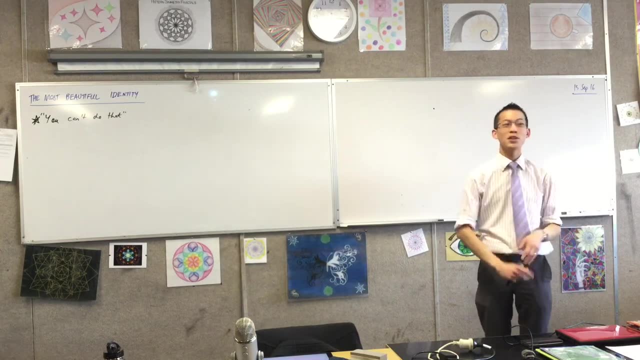 okay, Because we're going to go to some difficult places, but I promise it will be worth it, okay? Everyone in this room, regardless of how much maths I've been doing for the last two years, to understand this. okay, So I'm going to go right back to the beginning, okay, All? 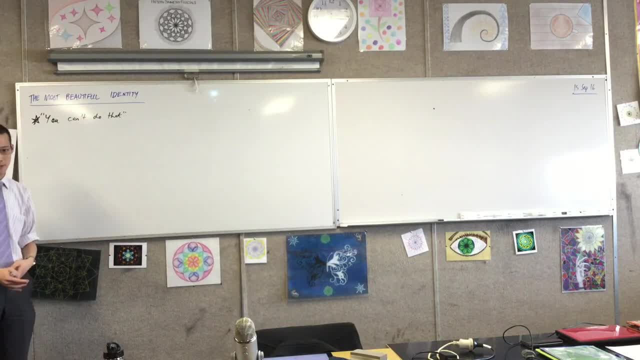 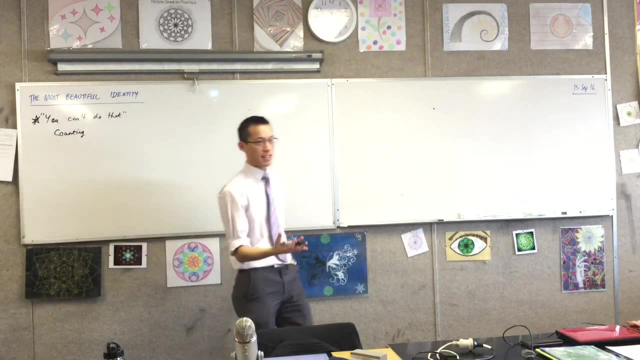 mathematics. in every culture throughout history, no matter where you are geographically, it always starts with the same idea, which is counting right, Even very, very young children have this concept of counting, so it's fairly sort of fundamental to the way we work and 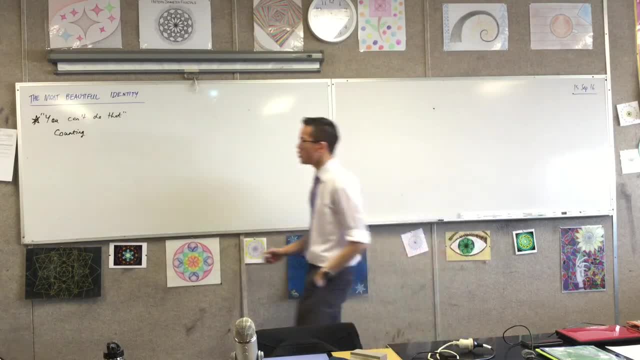 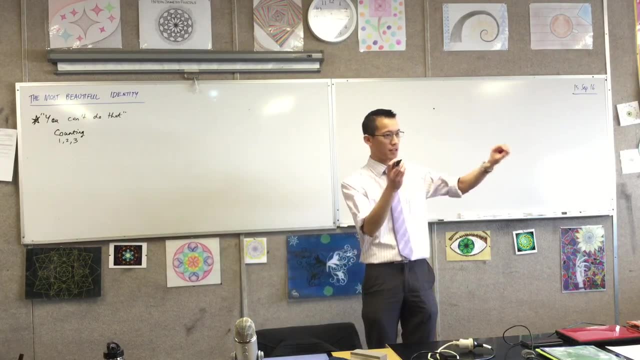 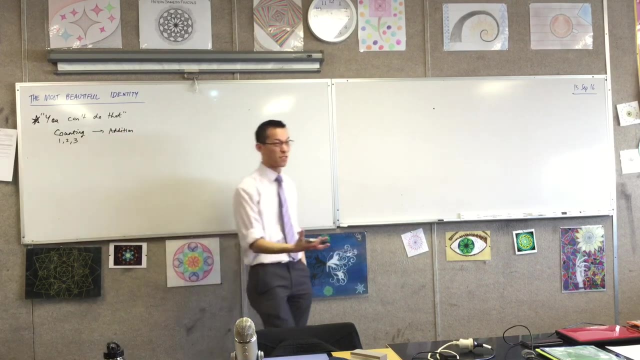 the way we sort of understand and interpret the reality around us. okay, So you start with counting, but as soon as you develop counting, It's fairly intuitive to move on from there to addition right, Like addition is actually. it begins just kind of as an extension of counting. right, You're plus 1, plus 1, plus. 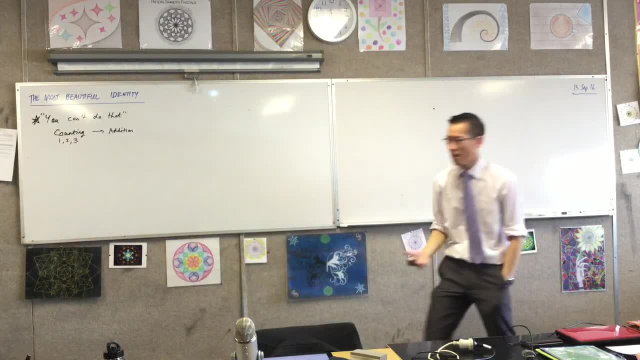 1,. and then you're like: well, why can't I add bigger numbers than that, right? So we can write something like: oh, I don't know, 11 plus 6 equals 17.. So addition comes out. 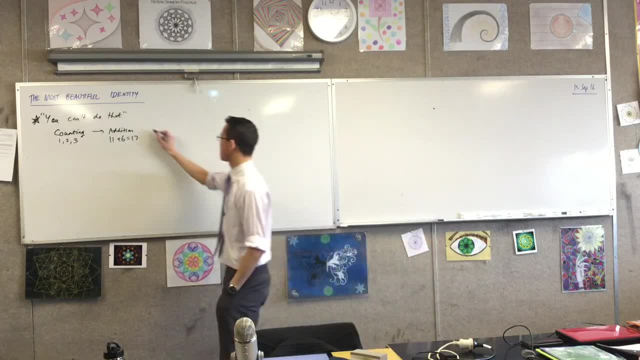 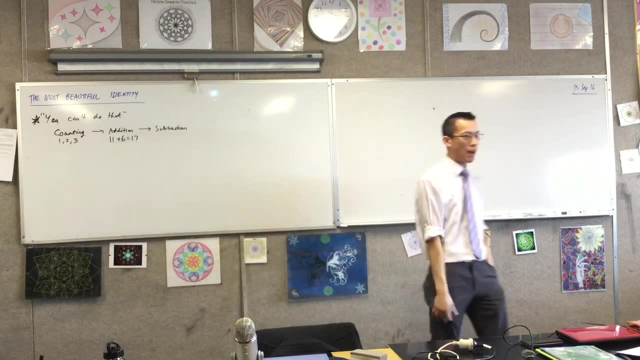 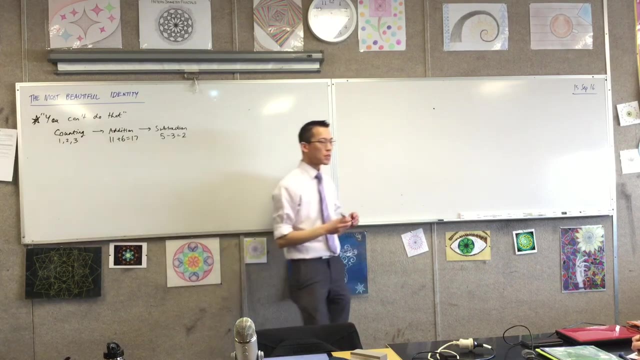 naturally. and then, as soon as you have addition, you have subtraction right, So you can put things onto a pile and you can take them away, and that's what subtraction is right. So we can write something like: 5, take away 3 equals 2.. Now, despite how little, 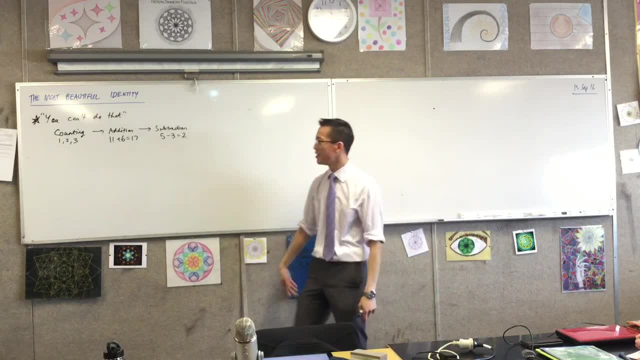 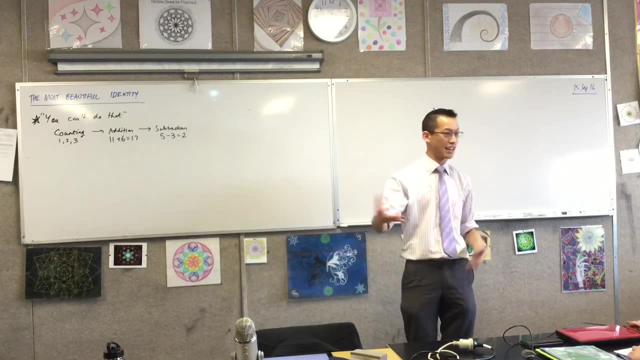 of a distance we have gone in terms of like mathematical concepts. okay, Counting and addition are incredibly free things. There are no rules really for counting an issue. You can count anything you like. In fact, that's one of the most amazing things about. 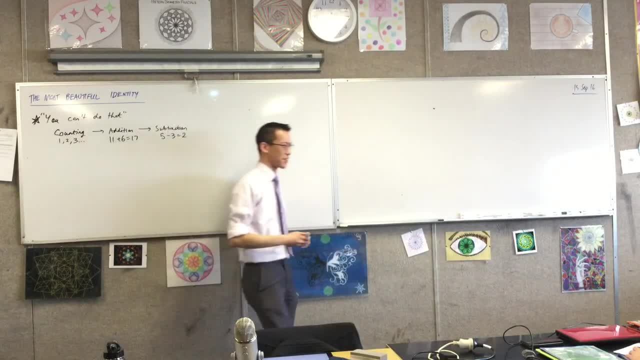 counting that. you know little kids. when they're like what's the biggest number you can think of? And they're like oh, 100. And you're like it's 101. And they're like oh. 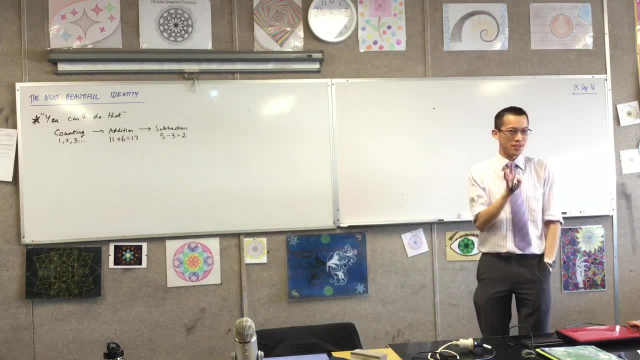 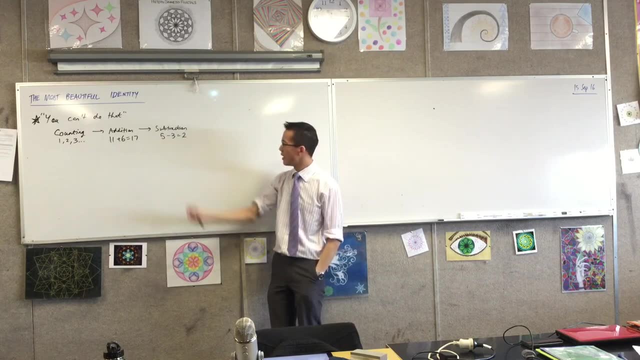 100, right, And you can keep on blowing up people's minds. There's no rules to do with what you can and can't count. And it's the same with addition: right, But the second you hit subtraction. this is the first moment when, suddenly, you will give something to a 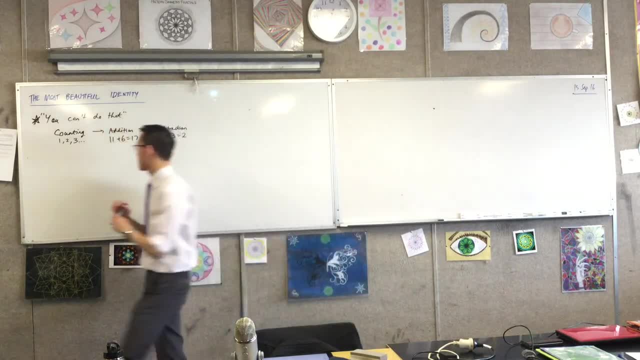 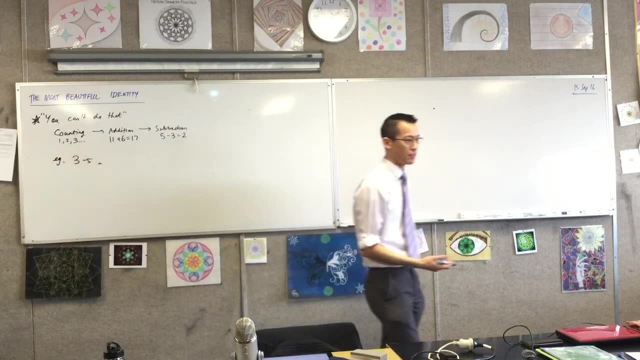 child and they'll say: oh, you can't do that right. For instance, you can't do this right. If you give this to a young enough child. you say, what's 3 take away 5?? They'll say: 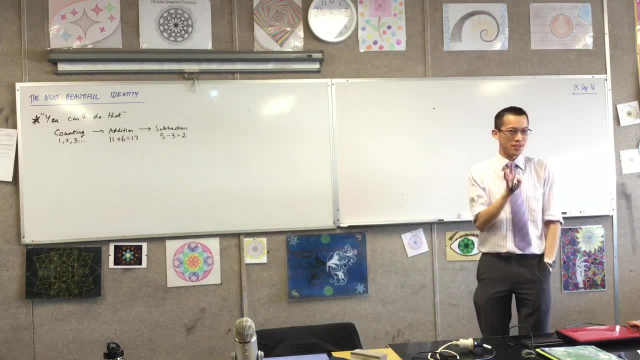 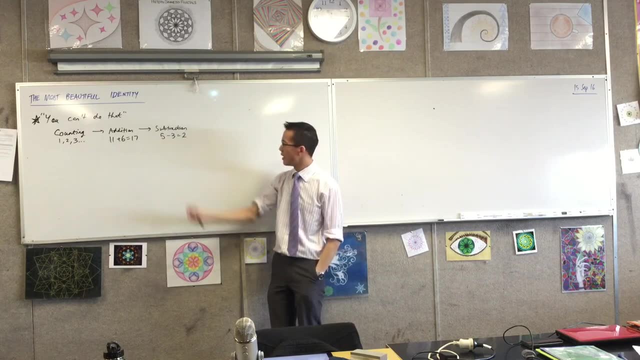 100, right, And you can keep on blowing up people's minds. There's no rules to do with what you can and can't count. And it's the same with addition: right, But the second you hit subtraction. this is the first moment when, suddenly, you will give something to a 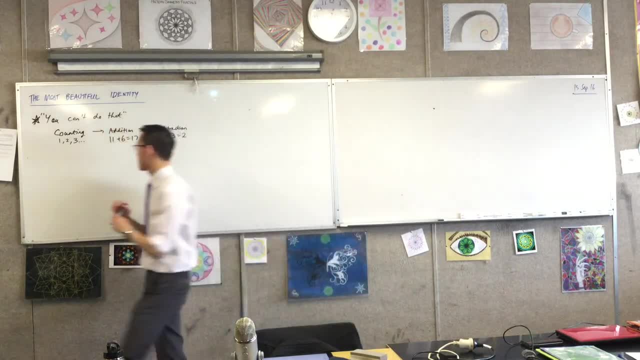 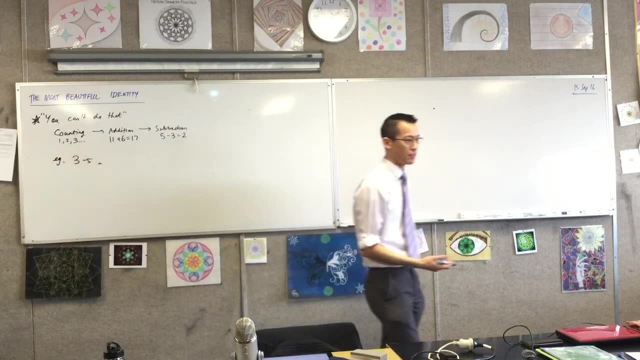 child and they'll say: oh, you can't do that right. For instance, you can't do this right. If you give this to a young enough child. you say, what's 3 take away 5?? They'll say: 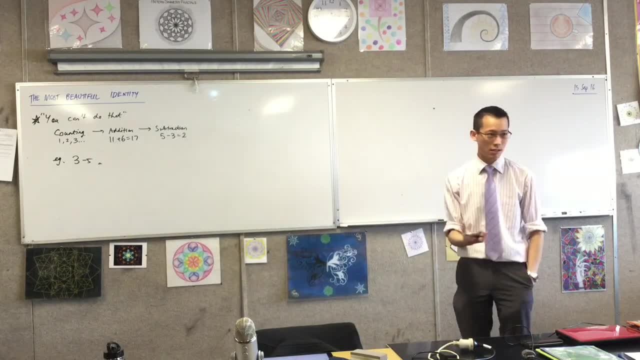 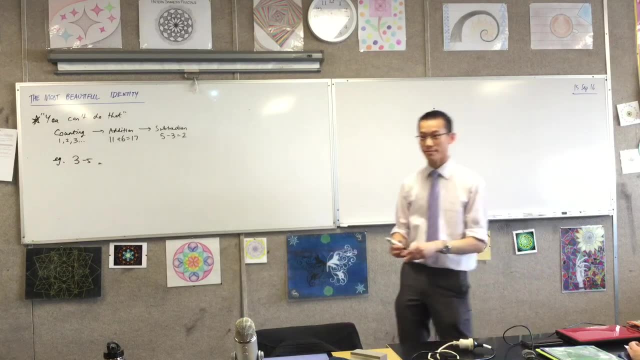 you can't do that. That's their response. right, Think It's not that crazy. I know it's been a long time since you've got that, but why can't you do 3 take away 5?? Yeah, there are only 3 objects there. I know what. 5 take away 3. 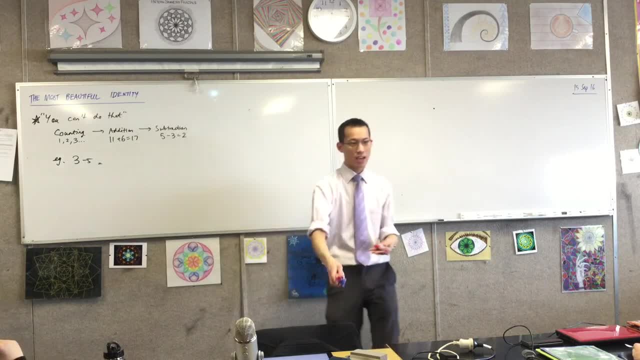 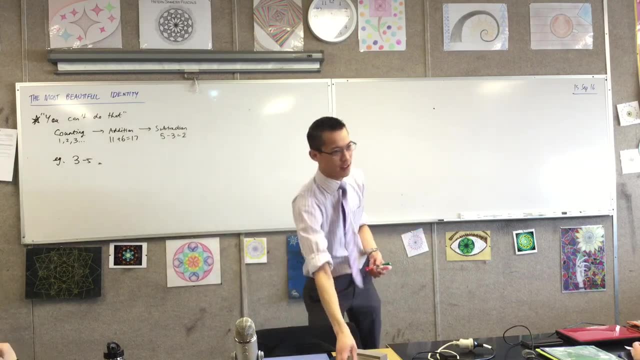 means It means you have 5 things and then you take away 3 of them. so that's what you get left with right. But if you reverse it, you're like, well, I've got 3 things and 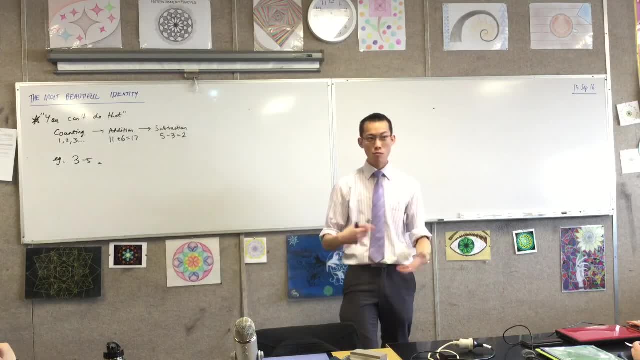 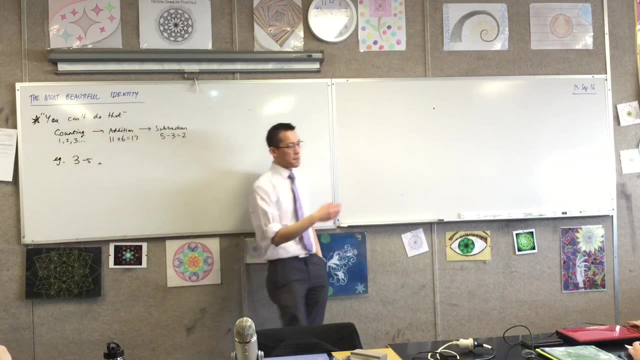 then I take away 1,, then I take away 2,, then I take away 3, and there are no more things to take away. okay, So when they say you can't do that, what we really mean is: I can't. 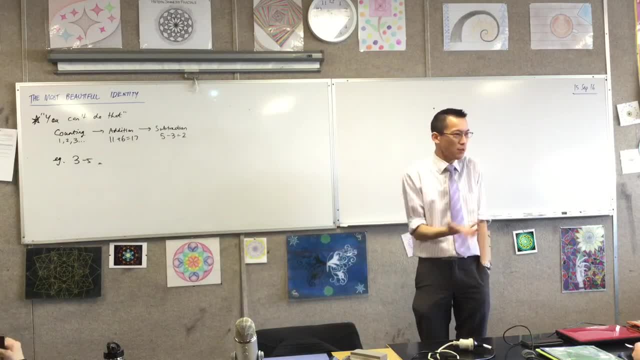 imagine a number. that would be a meaningful, sensible answer to this question. right, I don't have that number in my head. And then eventually we learn. Actually, you can imagine a whole family of numbers, a whole category of numbers. that's the answer to a question. 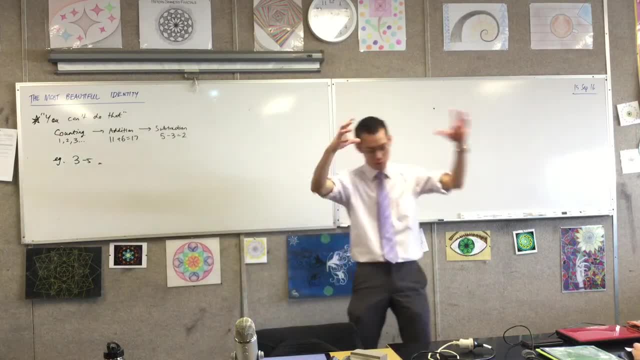 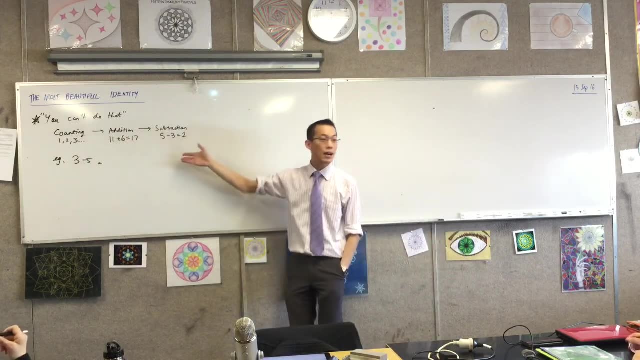 like this, right, And we call them negative numbers. and we say, okay, well, if you include these with the other ones, we call them integers, et cetera. okay, Now, all the way through, as we progress through mathematical concepts, we encounter problems. 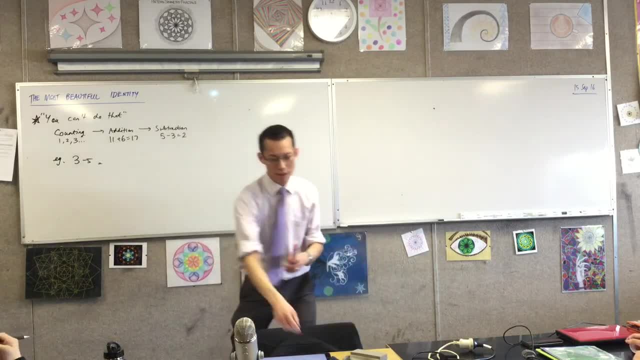 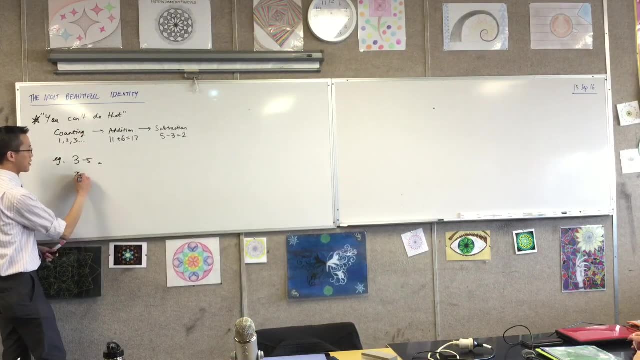 like this, right, So this kind of problem, right, I might phrase it slightly differently. I might phrase it in terms of, like an equation you have to solve, okay, So if I said to you x plus 3 equals 0, right, Like, try and tell me the number that if you add 3 to it, you 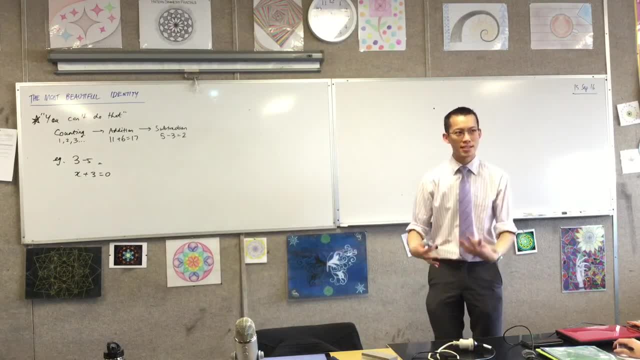 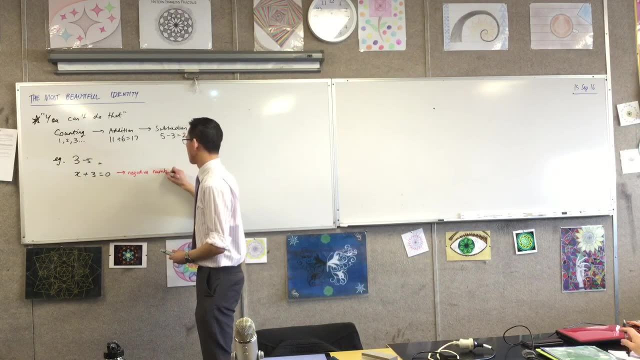 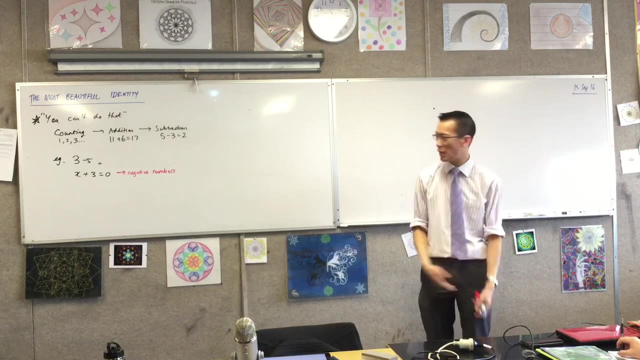 get 0,. okay, Try to solve this equation, sort of necessitate. okay, I need something called negative numbers, right, And I don't want you to, I don't want you to miss. negative numbers were a crazy idea for centuries. People were like, well, you can't measure them right. It's like this: 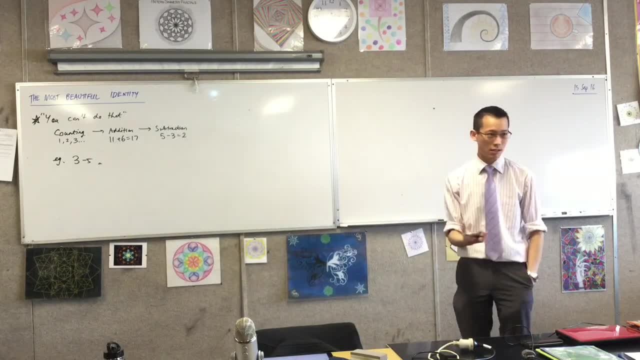 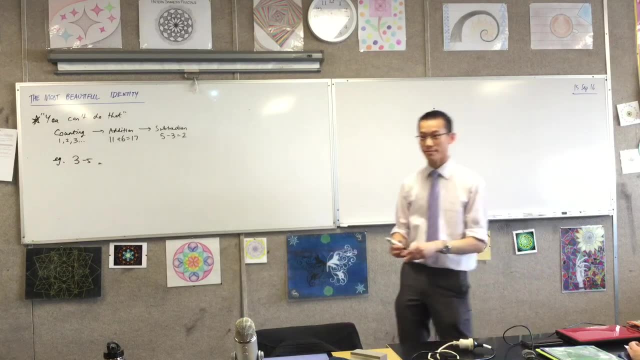 you can't do that. That's their response. right, Think It's not that crazy. I know it's been a long time since you've got that, but why can't you do 3 take away 5?? Yeah, there are only 3 objects there. I know what. 5 take away 3. 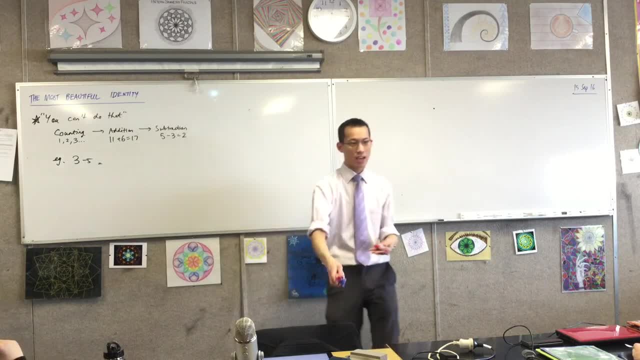 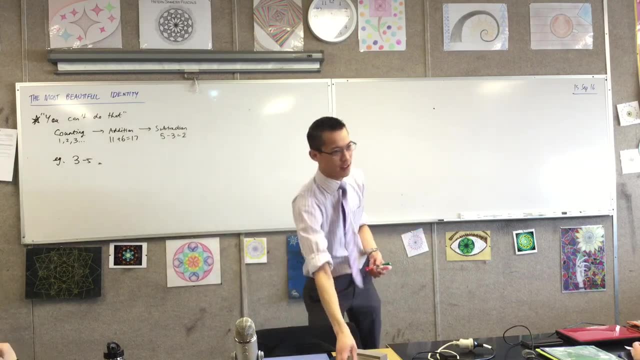 means It means you have 5 things and then you take away 3 of them. so that's what you get left with right. But if you reverse it, you're like, well, I've got 3 things and 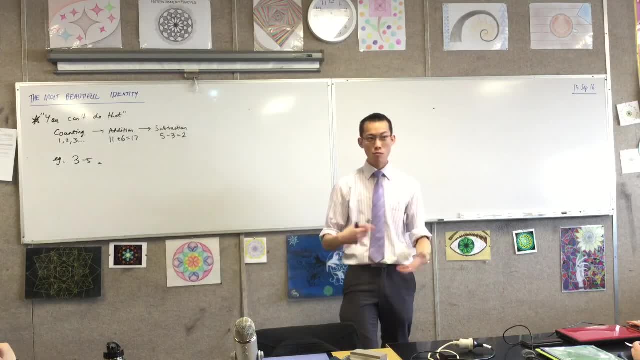 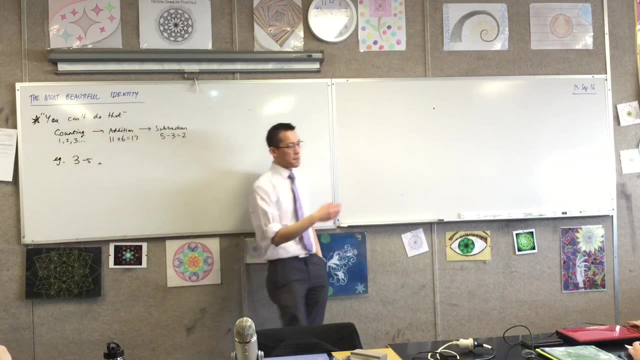 then I take away 1,, then I take away 2,, then I take away 3, and there are no more things to take away. okay, So when they say you can't do that, what we really mean is: I can't. 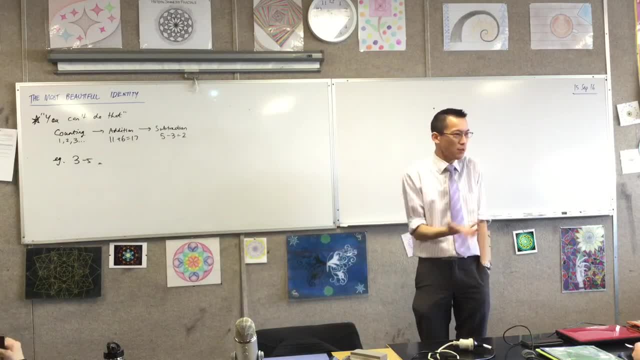 imagine a number. that would be a meaningful, sensible answer to this question. right, I don't have that number in my head. And then eventually we learn. Actually, you can imagine a whole family of numbers, a whole category of numbers. that's the answer to a question. 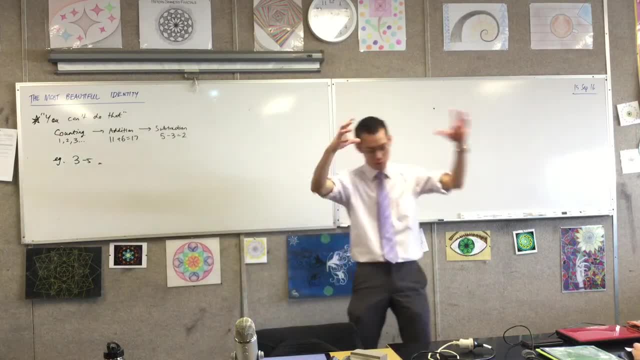 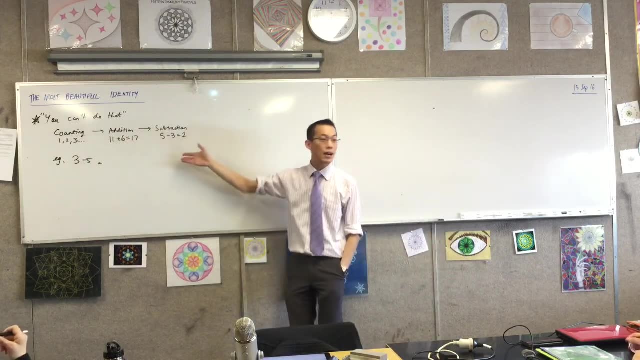 like this, right, And we call them negative numbers. and we say, okay, well, if you include these with the other ones, we call them integers, et cetera. okay, Now, all the way through, as we progress through mathematical concepts, we encounter problems. 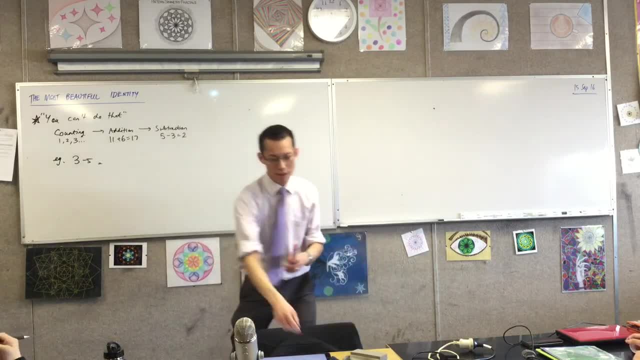 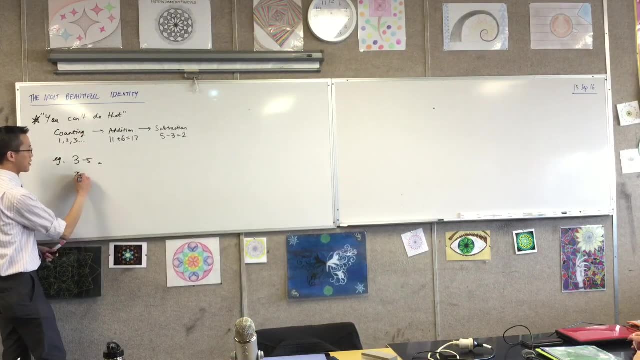 like this, right, So this kind of problem, right, I might phrase it slightly differently. I might phrase it in terms of, like an equation you have to solve, okay, So if I said to you x plus 3 equals 0, right, Like, try and tell me the number that if you add 3 to it, you 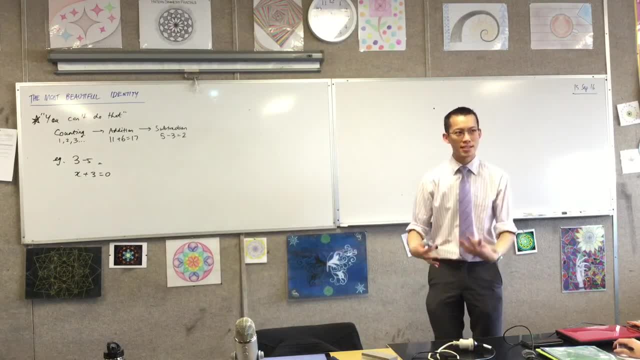 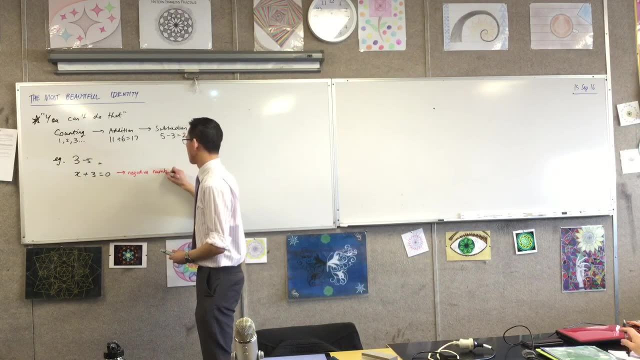 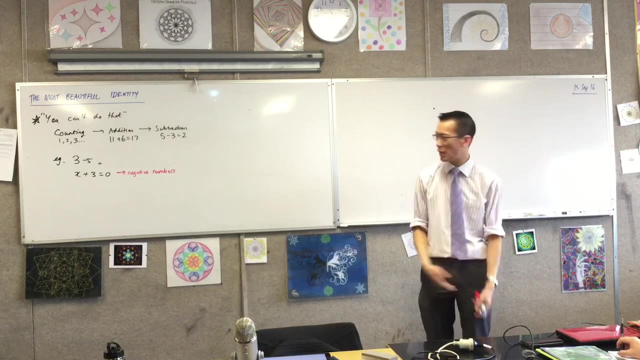 get 0,. okay, Try to solve this equation, sort of necessitate. okay, I need something called negative numbers, right, And I don't want you to, I don't want you to miss. negative numbers were a crazy idea for centuries. People were like, well, you can't measure them right. It's like this: 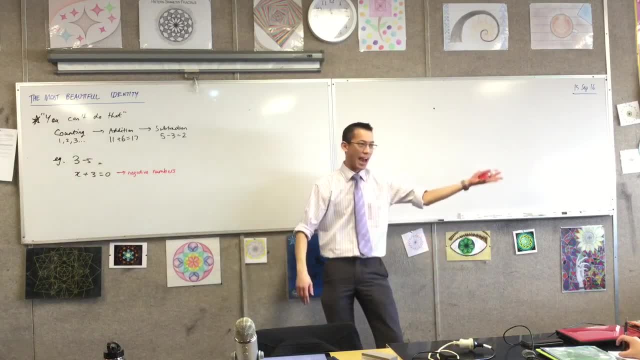 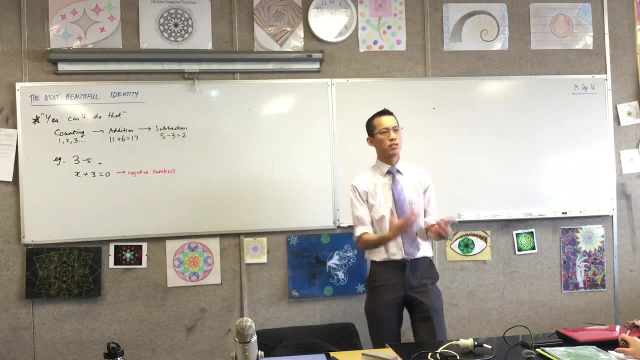 table can be this by this, but you can't say it's negative this or I can't have negative cows or whatever. right, It doesn't make sense in a counting scheme. But this isn't the only time that this kind of thing has happened, that we've had to imagine a new way of thinking. 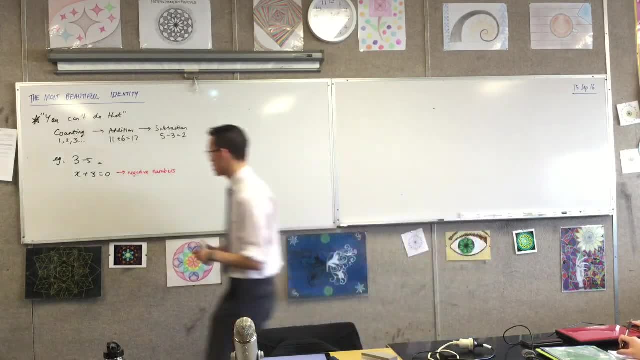 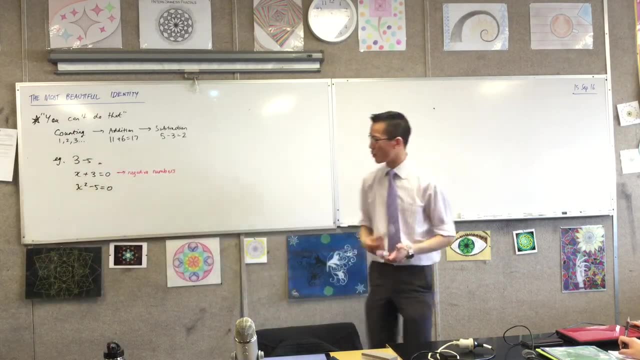 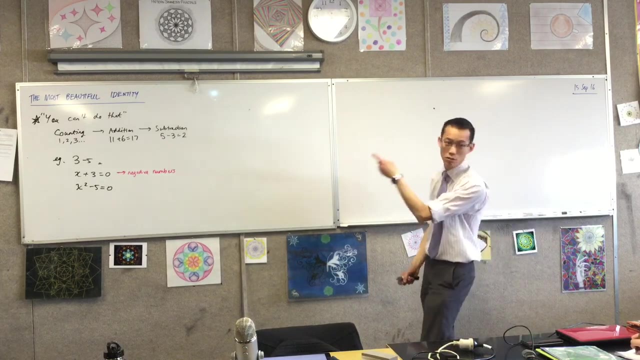 about numbers because of a kind of problem we've tried to solve. For instance, here's another one. If you went to an ancient Greek right, they would have said: well, you can't do that, you can't do that because there's no number. they could imagine that would be a suitable 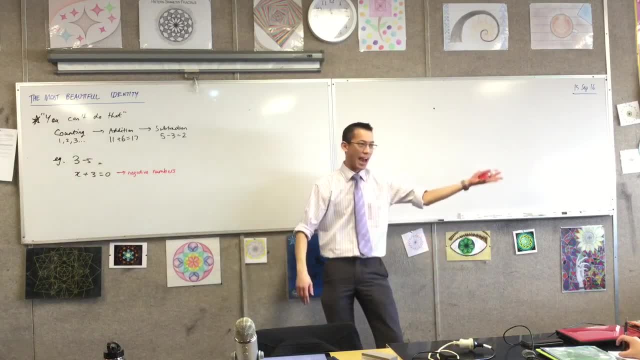 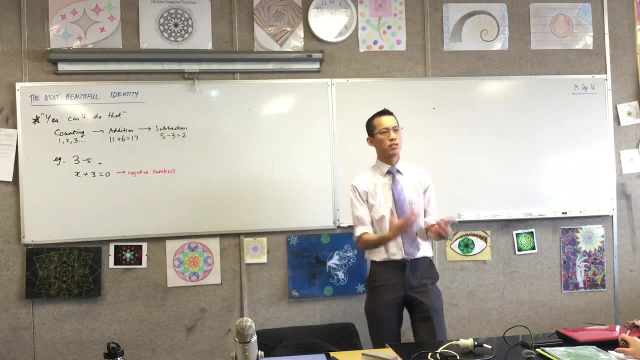 table can be this by this, but you can't say it's negative this or I can't have negative cows or whatever. right, It doesn't make sense in a counting scheme. But this isn't the only time that this kind of thing has happened, that we've had to imagine a new way of thinking. 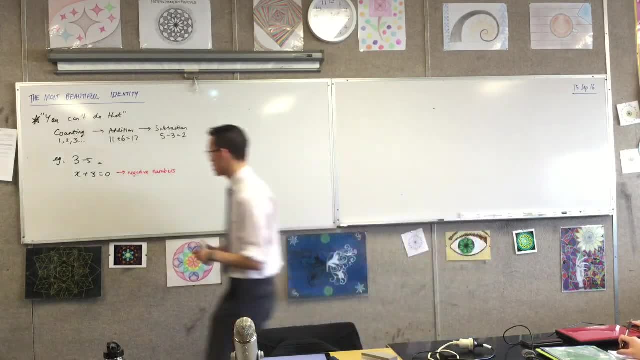 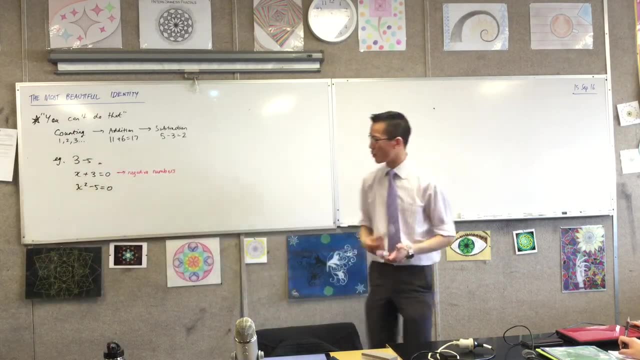 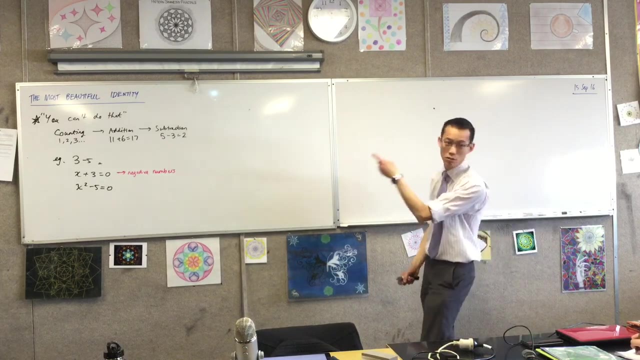 about numbers because of a kind of problem we've tried to solve. For instance, here's another one. If you went to an ancient Greek right, they would have said: well, you can't do that, you can't do that because there's no number. they could imagine that would be a suitable 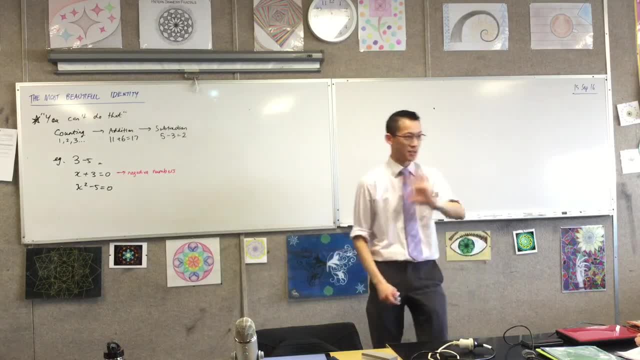 solution to this equation. right, They would think of fractions until they were blue in the face, and no fraction will do it. right, No fraction will do it. And so they said: well, if there are no numbers that are rational, that are a ratio between two things, we need. 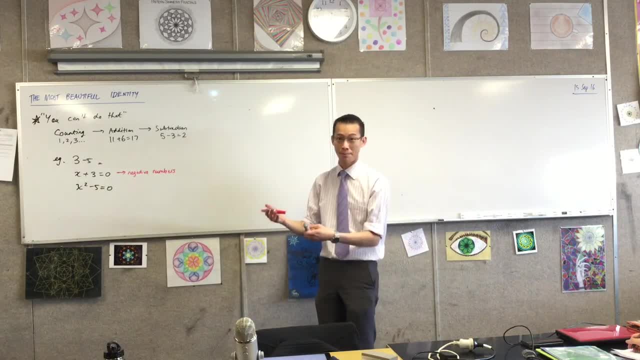 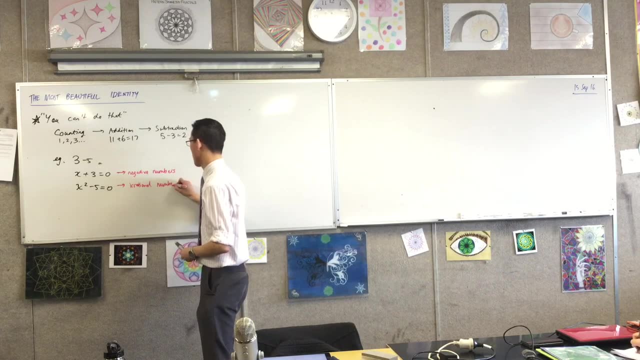 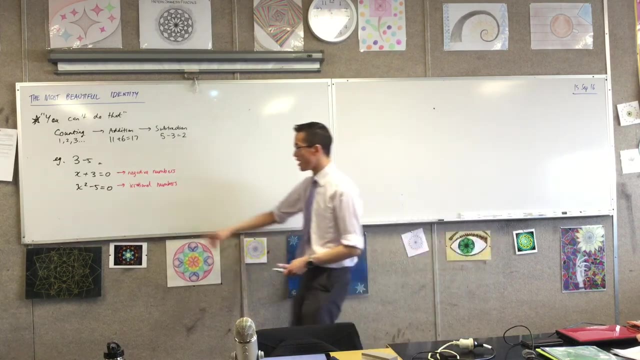 to imagine a new family, a new category of numbers, and we call them irreversible numbers, Irrational numbers. Now I should say, just like with negative numbers, that these numbers were considered just nonsensical for centuries, right, And that is why the word irrational. 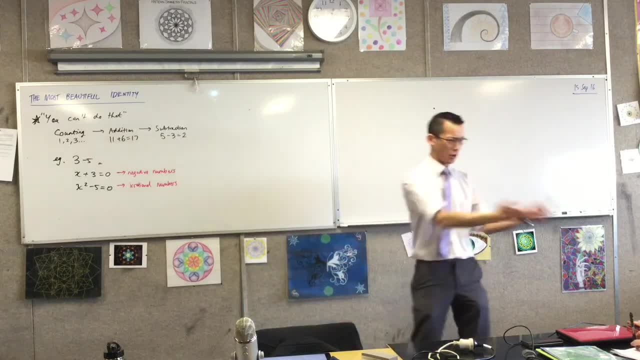 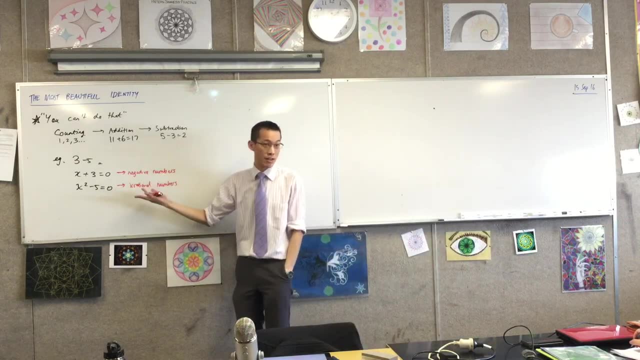 literally in our language, means nonsensical. when you say: stop being irrational, right, It's a holdover from the time when this idea, like we know this, means not ratio. You can't write it as a ratio. right, The square root of five. okay, It's a third, We have a whole. 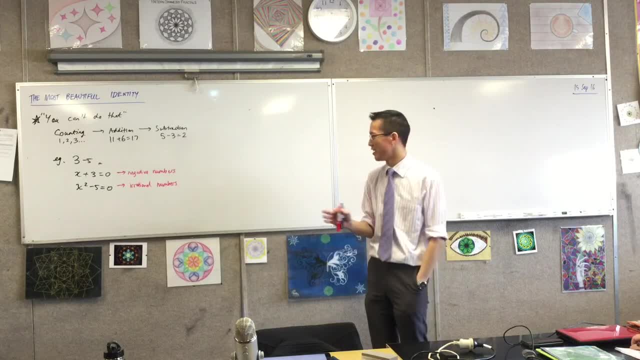 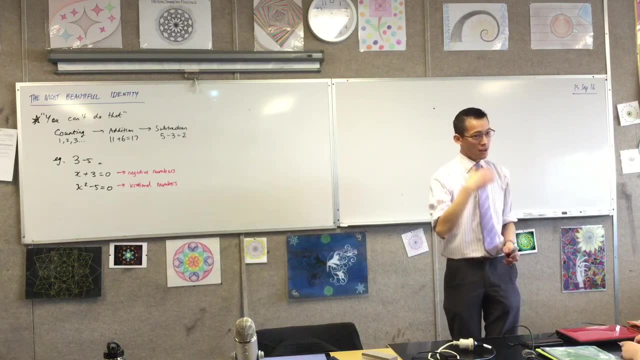 new category of things for this right, But because it was such a crazy idea, this word, which means not a ratio, came to mean it doesn't make sense. okay, Now, this has happened many more times, but the time I'm 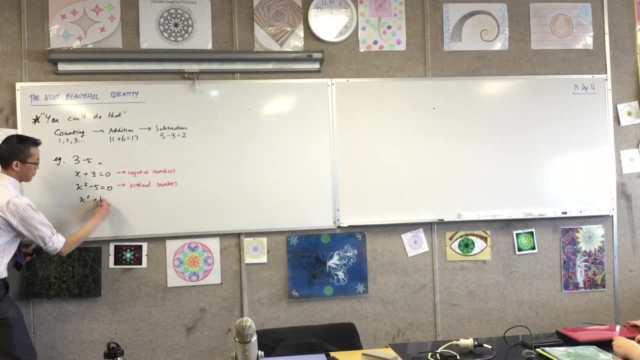 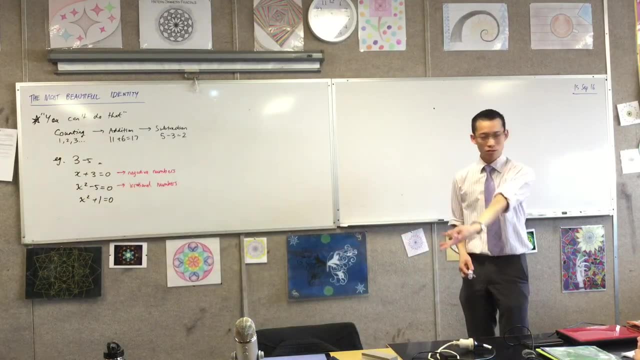 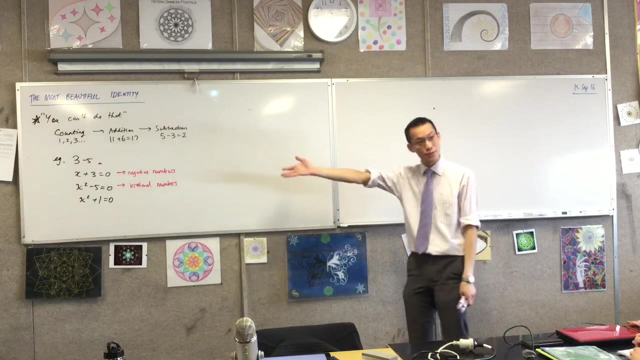 most interested in for an equation is this guy. Okay, you can add negatives, you can have irrational numbers, but no negative numbers, no irrational numbers will solve this equation. We can't imagine this concept right of what kind of number would be a suitable, meaningful? 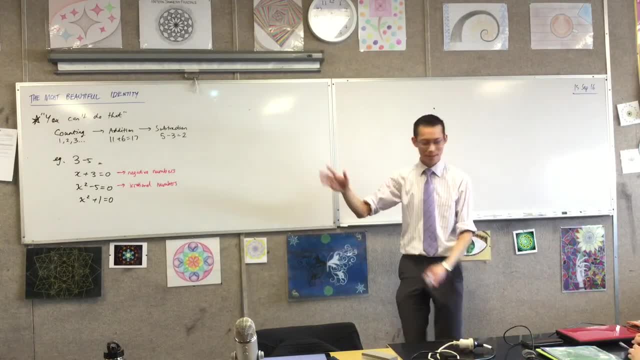 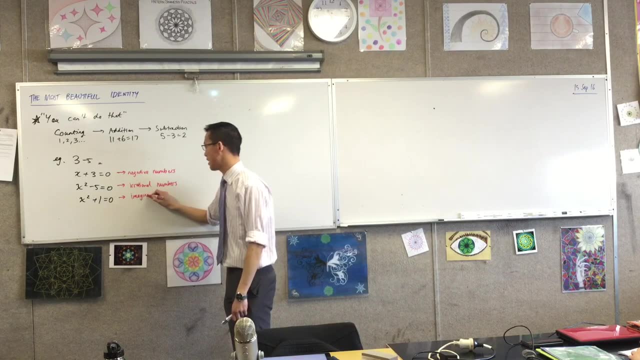 answer to this right, And I've been dropping the word imagine on purpose, because the category of numbers that we fashion, invented, are called imaginary numbers. Again, getting sick of hearing this. probably this is a derogatory term right which was fashioned by the people. 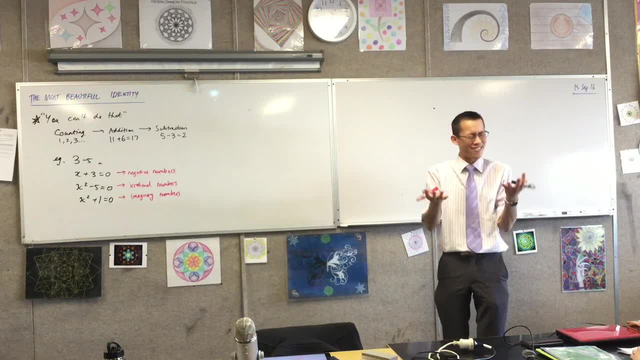 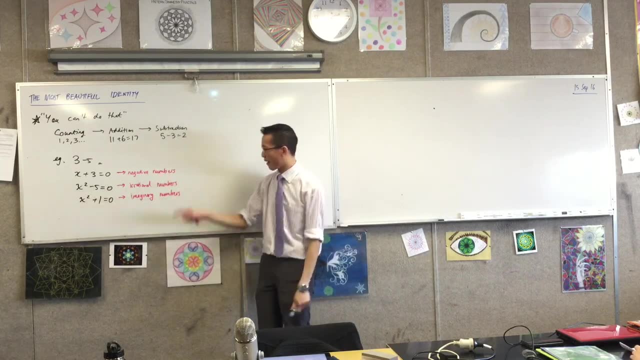 who opposed the idea of this and they said: these numbers aren't real. Where are they in nature? Where can you find these? At least, I can talk about these as, like you know, backwards and forwards, or I can think about these on like, on the hypotenuse of a of. 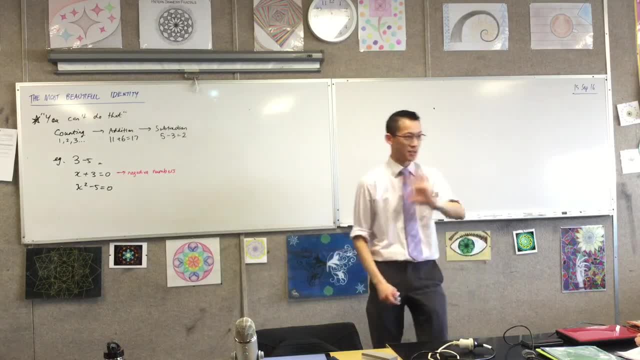 solution to this equation. right, They would think of fractions until they were blue in the face, and no fraction will do it. right, No fraction will do it. And so they said: well, if there are no numbers that are rational, that are a ratio between two things, we need. 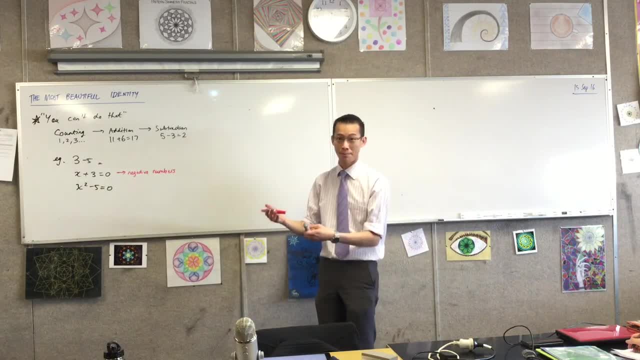 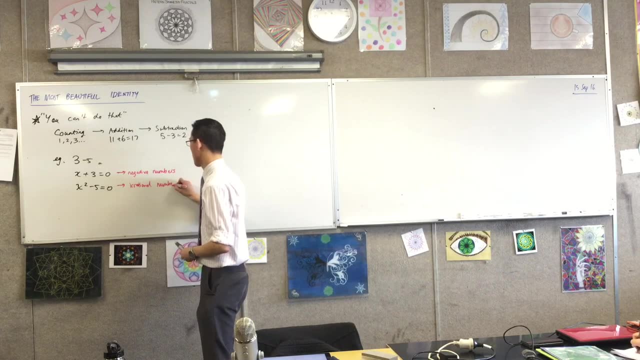 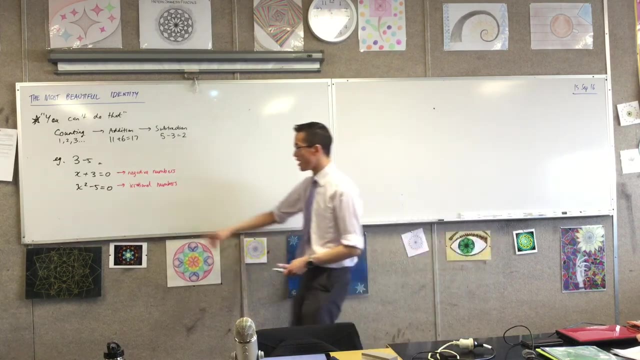 to imagine a new family, a new category of numbers, and we call them irreversible numbers, Irrational numbers. Now I should say, just like with negative numbers, that these numbers were considered just nonsensical for centuries, right, And that is why the word irrational. 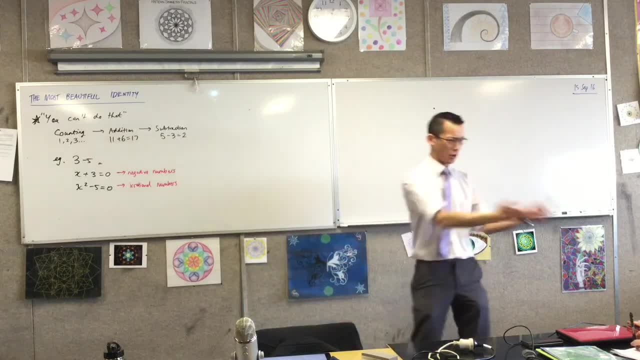 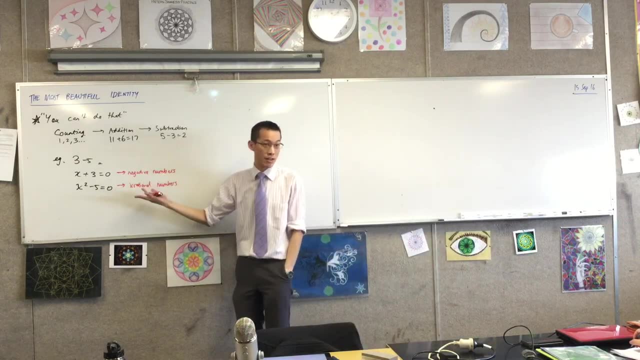 literally in our language, means nonsensical. when you say: stop being irrational, right, It's a holdover from the time when this idea, like we know this, means not ratio. You can't write it as a ratio. right, The square root of five. okay, It's a third, We have a whole. 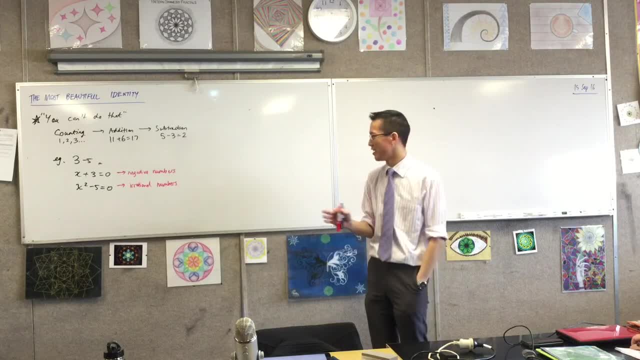 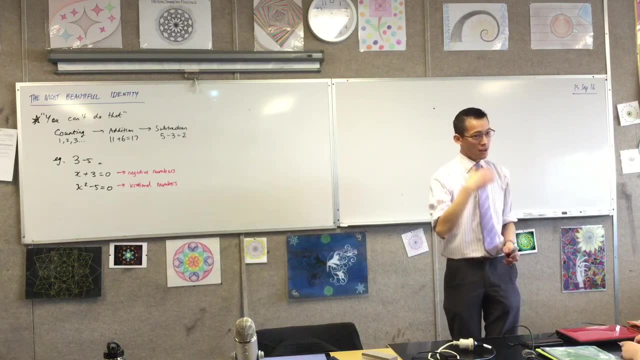 new category of things for this right, But because it was such a crazy idea, this word, which means not a ratio, came to mean it doesn't make sense. okay, Now, this has happened many more times, but the time I'm 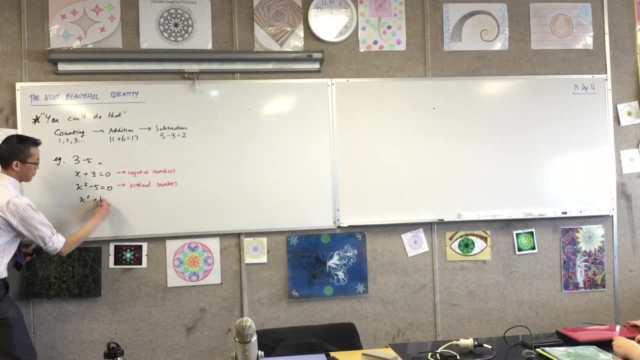 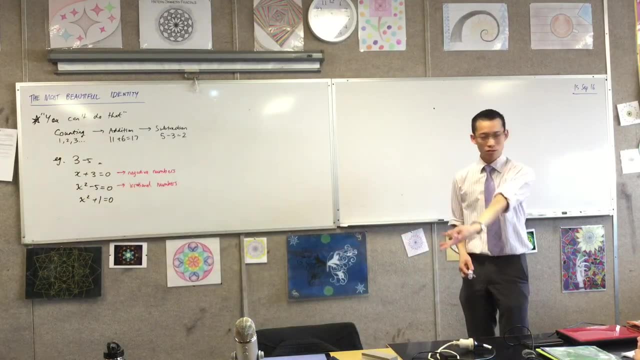 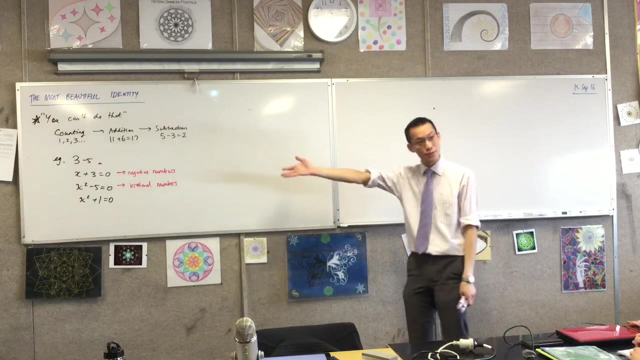 most interested in for an equation is this guy. Okay, you can add negatives, you can have irrational numbers, but no negative numbers, no irrational numbers will solve this equation. We can't imagine this concept right of what kind of number would be a suitable, meaningful? 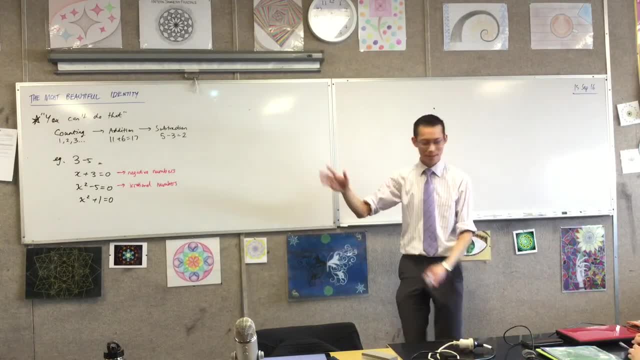 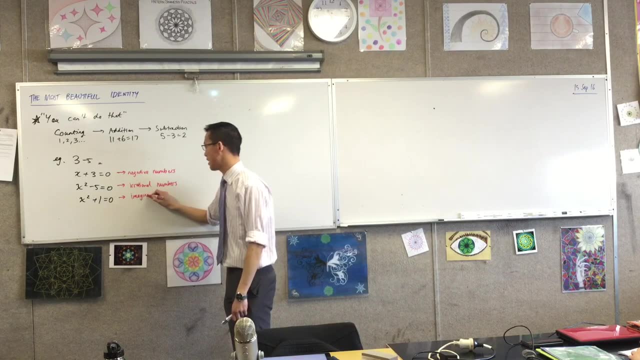 answer to this right, And I've been dropping the word imagine on purpose, because the category of numbers that we fashion, invented, are called imaginary numbers. Again, getting sick of hearing this. probably this is a derogatory term right Which was fashioned by the people. 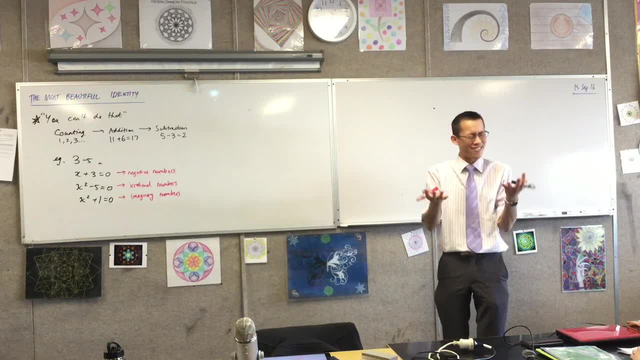 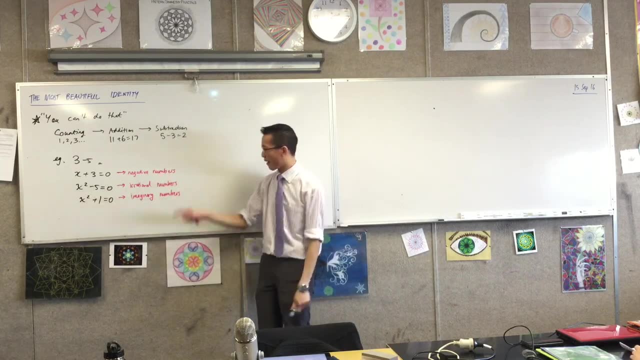 who opposed the idea of this and they said: these numbers aren't real. Where are they in nature? Where can you find these? At least, I can talk about these as, like you know, backwards and forwards, or I can think about these on like, on the hypotenuse of a of. 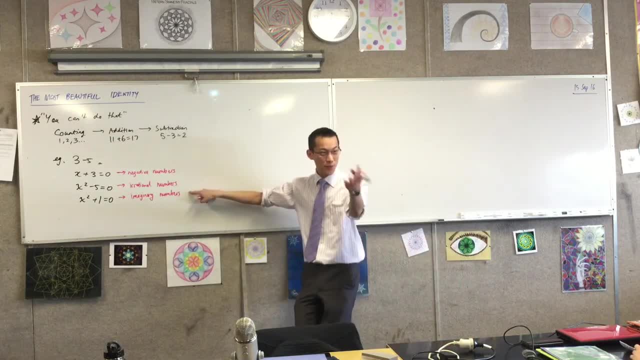 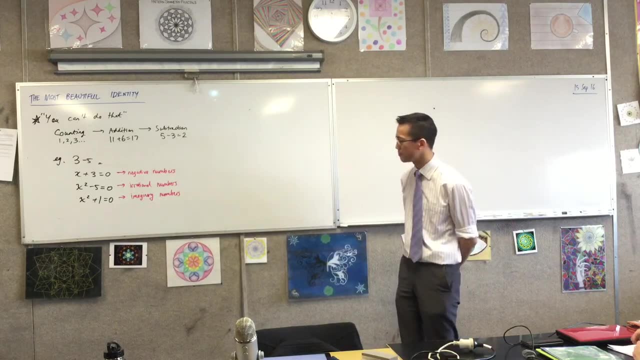 a right angle triangle. Where are you going to find these? Huh, Go, look, go, look for them and tell me where they are. They're not real And so they were called imaginary numbers, because you can't measure them, you can't see them, all that kind of thing. okay, Now 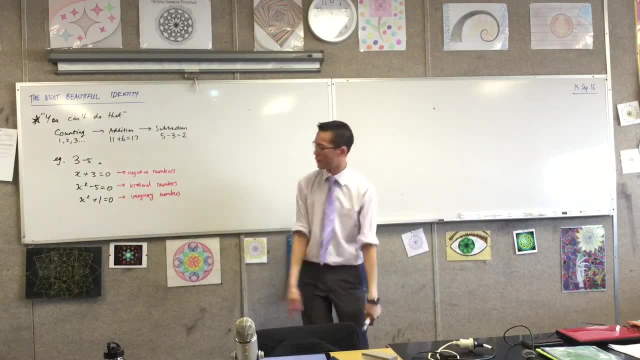 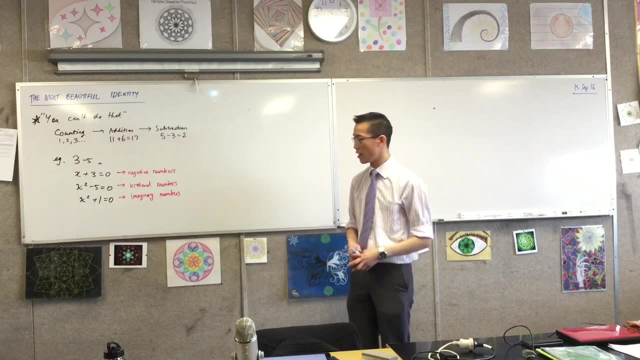 this particular equation is important because it's kind of like the building block of all of these. If I gave you x squared plus 3 or x squared plus 5 or x squared plus anything, all of them would be a version of this one, just bigger or smaller. okay, If we went ahead. 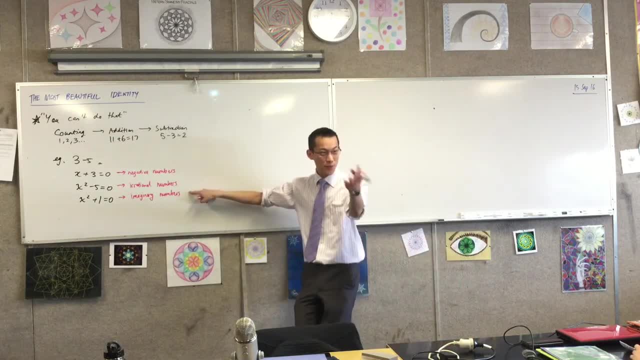 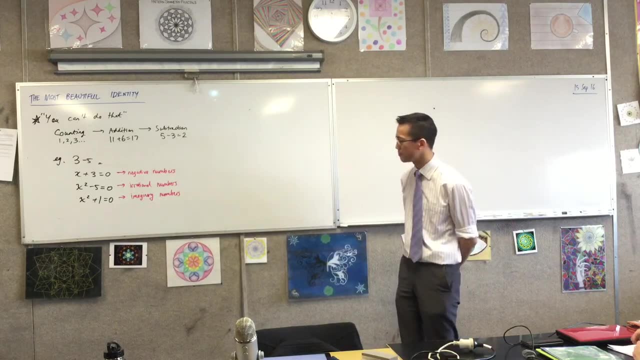 a right angle triangle. Where are you going to find these? Huh, Go, look, go, look for them and tell me where they are. They're not real And so they were called imaginary numbers, because you can't measure them, you can't see them, all that kind of thing. okay, Now 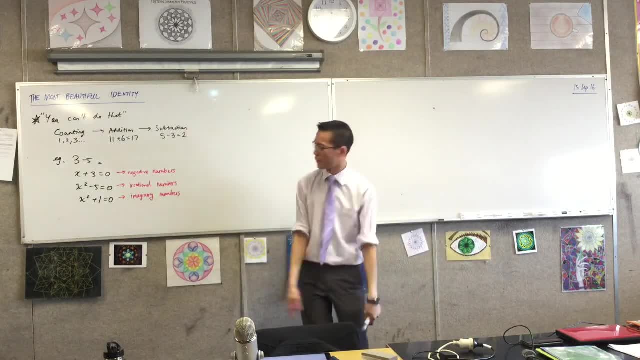 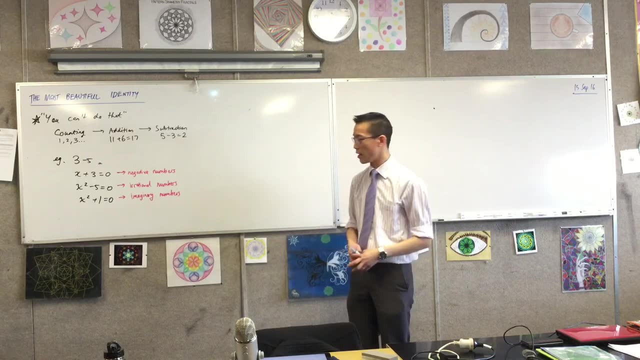 this particular equation is important because it's kind of like the building block of all of these. If I gave you x squared plus 3 or x squared plus 5 or x squared plus anything, all of them would be a version of this one, just bigger or smaller. okay, If we went ahead. 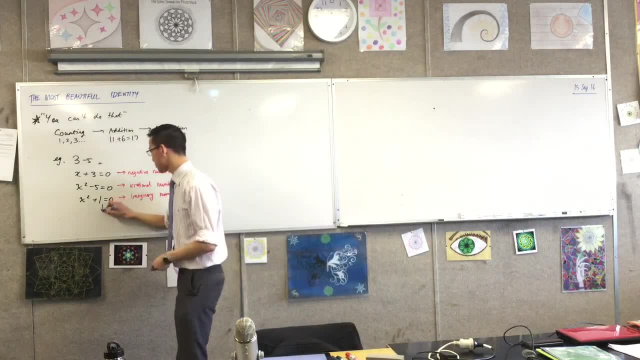 and solved this. let's get this down with me: You should have all three of these, really. If I take this, x squared plus 1, right, It's like? well, just do the non-negotiable, right, You should have all three of these, really. If I take this, x squared plus 1, right It's. 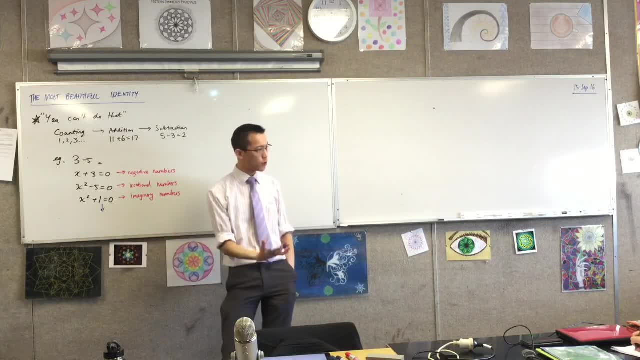 like, well, just do the non-negotiable right. It's like, well, just do the non-negotiable right. It's like, well, just do the non-negotiable right, Use all of your algebraic manipulation. 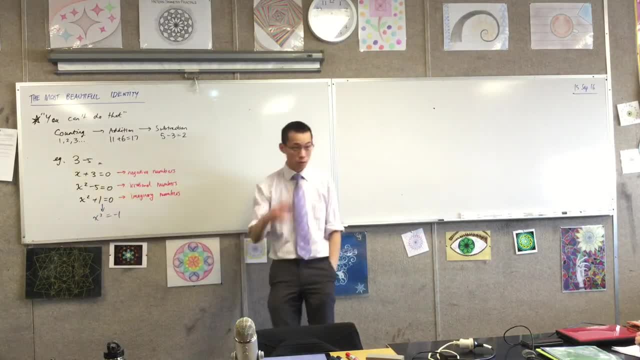 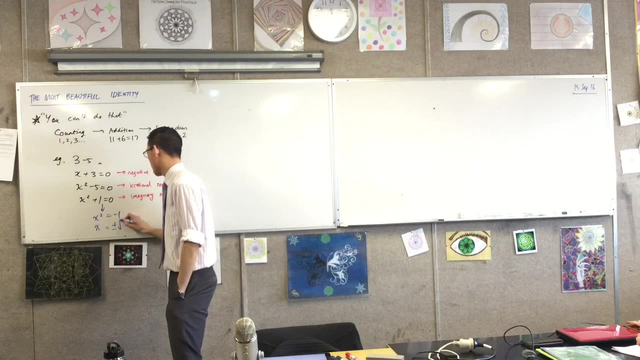 skills. You'd say: well, I want the x's on their own, So we'll get all the constants out of the way And you'll be like: well, I guess I take the square root of both sides now, right, And this is the point at which we say, oh, you can't do that, right. 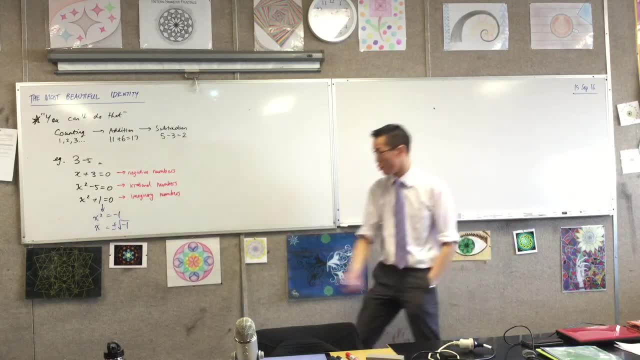 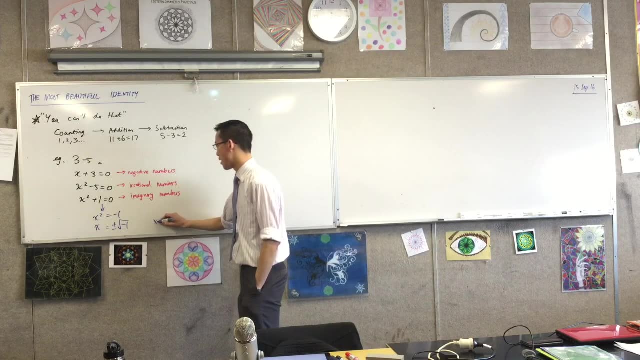 Unite and 10 and even 2 unit and extension 1u says you can't do that, but but what if you could? So we call this guy, we say uh, uh, uh uh. that the square root of negative 1, we give this a name. we call it after the name, right? 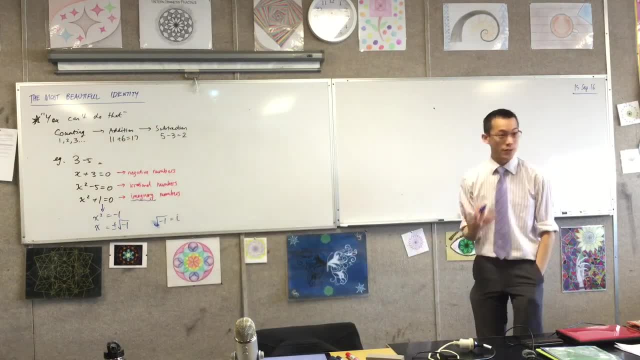 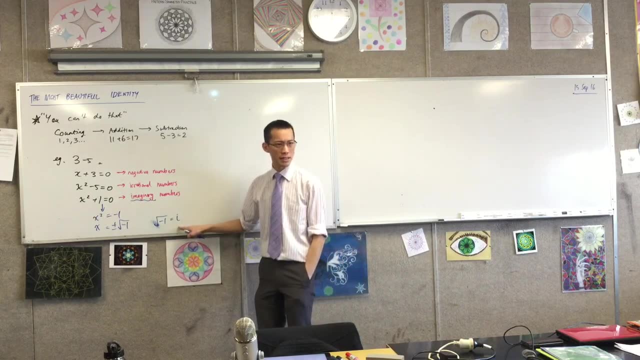 We call it: i okay Every square root of a negative number. okay, the square root of negative 5, right? or the square root of negative 16, they're just multiples of i right. Do you get that? Like, for example, if I said the square root of negative 16,. 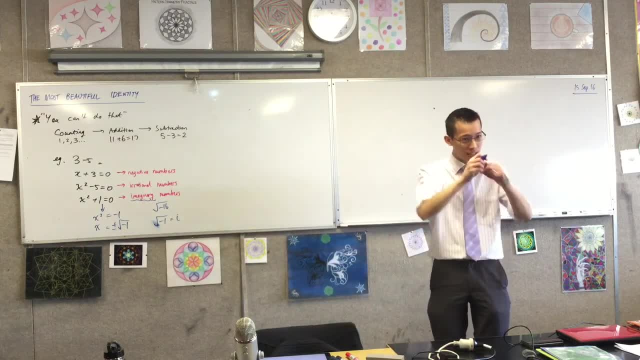 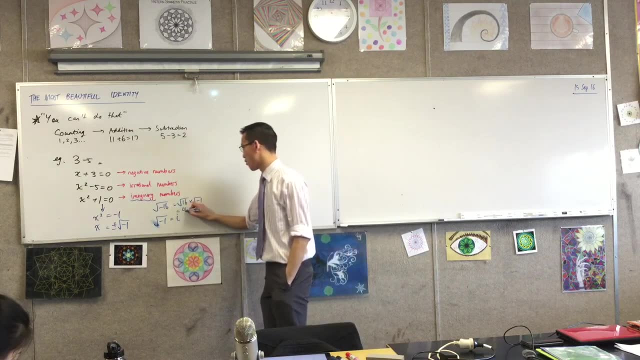 we can use some operations here to separate this out. This is root 16 times root negative 1, do you agree? Right? so that's 4 times the square root of negative 1, so that's 4i, okay. 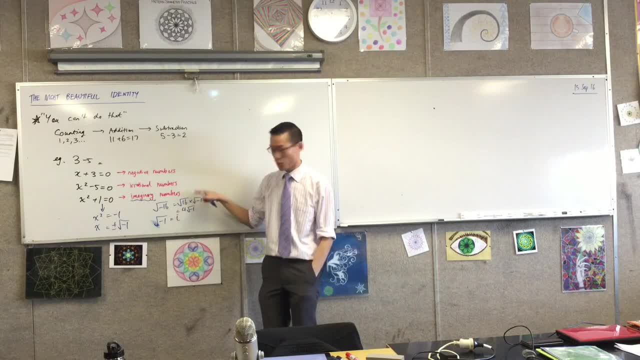 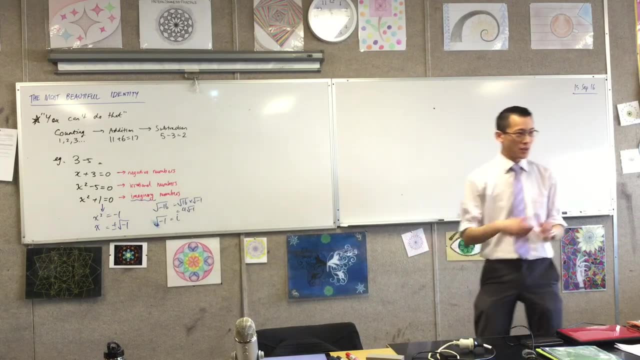 So this is just kind of like your basic building block. You don't need new names for all of these guys if they're all just bigger and smaller versions of the square root of negative 1, okay, All right. so here's this idea of you. can't do that. 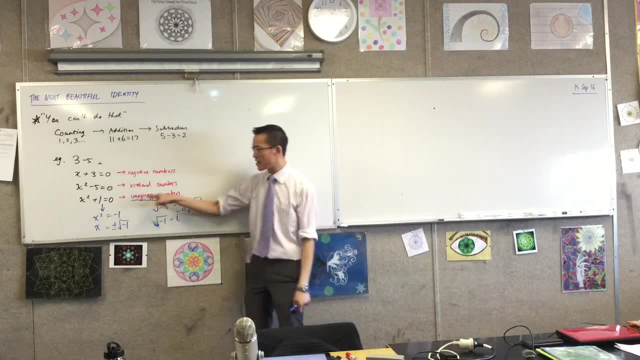 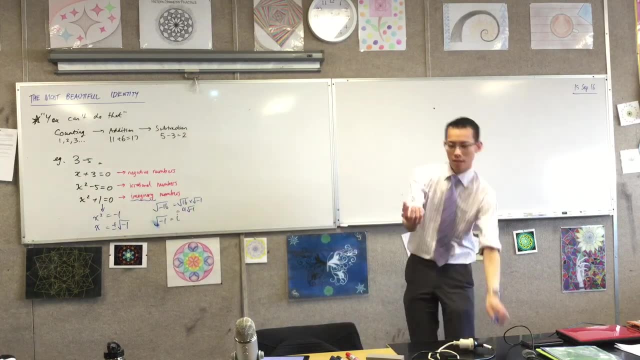 Well, what if you could? okay, Now we call these guys imaginary numbers. If you put them together with the numbers, you're already familiar with these negative numbers, irrational numbers, et cetera. they're actually kind of. They're kind of like oil and water, right? 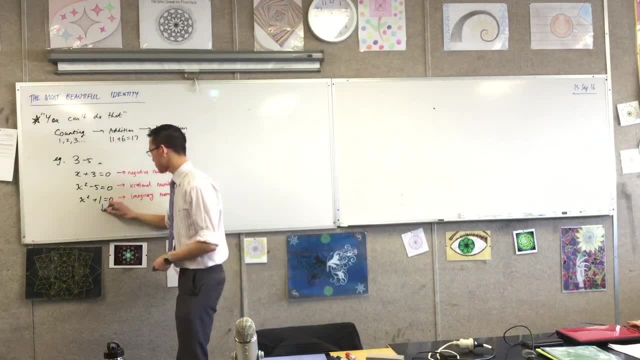 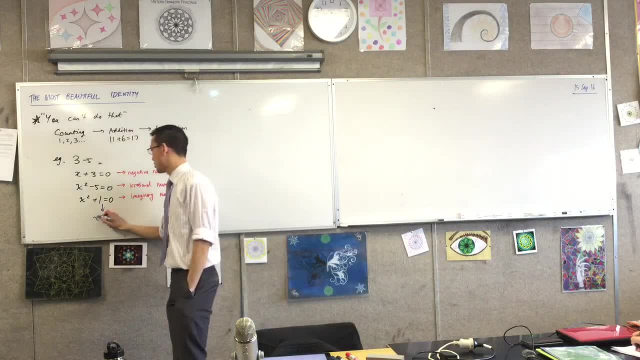 know they're the same thing, but when you do the normal thing that you would do when you're solving an equation like this, use all of your algebraic manipulation skills. you'd say: well, I want the x's on their own, So I'll get all of the constants out. 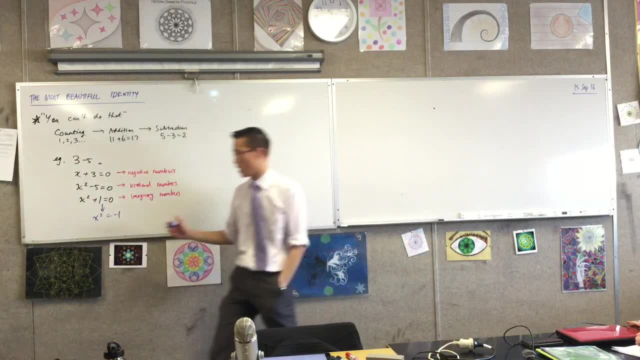 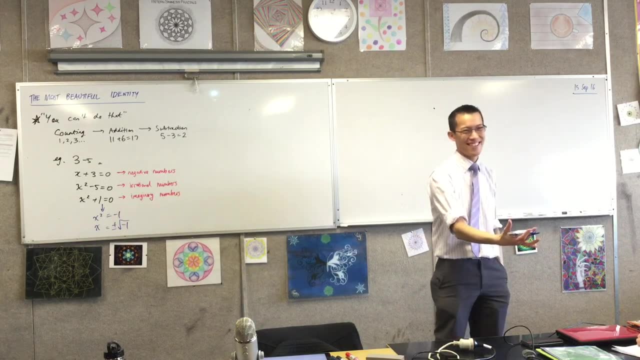 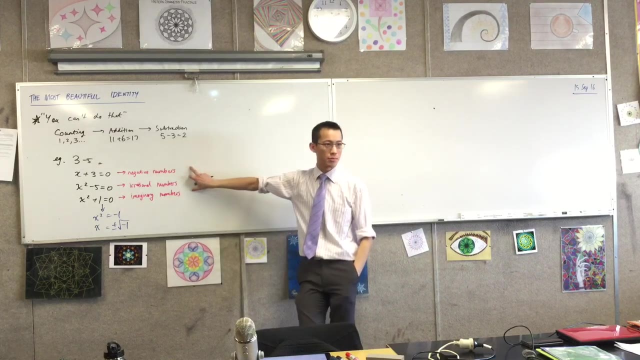 of the way. Then you say: well, I guess I take the square root of both sides. now, right, And this is the point at which we say, oh, you can't do that. right, Unit and 10, and even two unit and extension. one u says you can't do that, But what if you could? right. 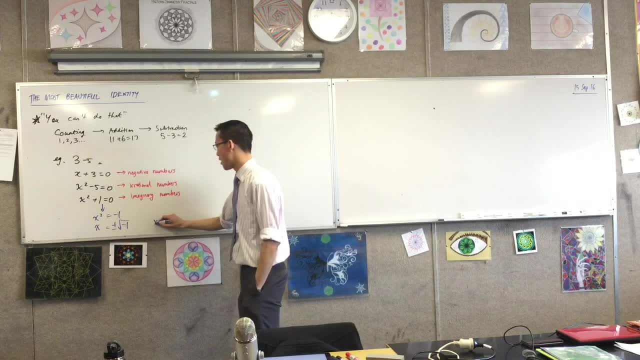 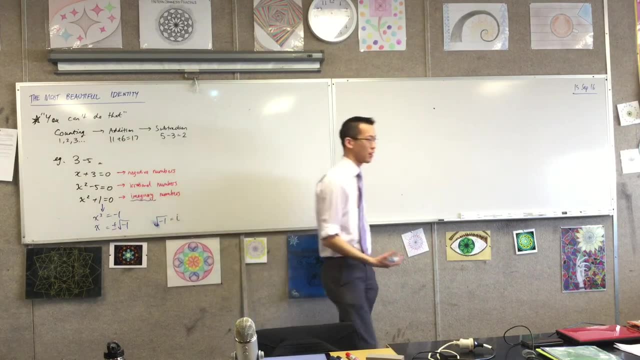 So we call this guy, we say that, the square root of negative 1,. we give this a name, we call it after the name, right, We call it. i okay. Every square root of a negative number, let's say the square root of negative 5, right. 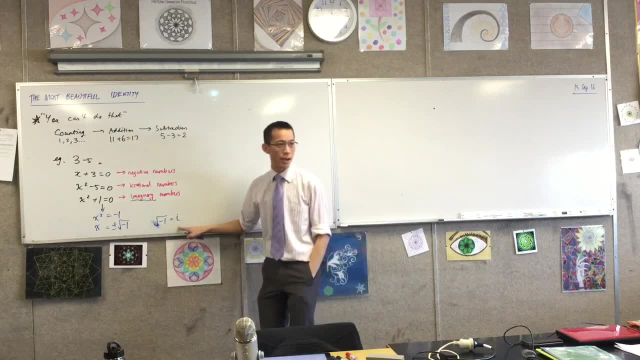 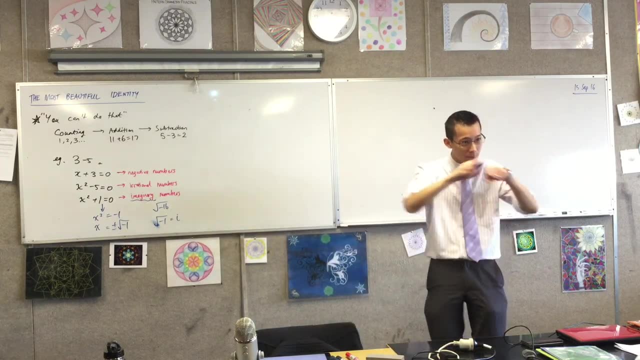 or the square root of negative 16, they're just multiples of, i right. Do you get that Like, for example, if I said the square root of negative 16, we can use some operations here to separate this out. Now, this is root 16 times root of negative 1.. 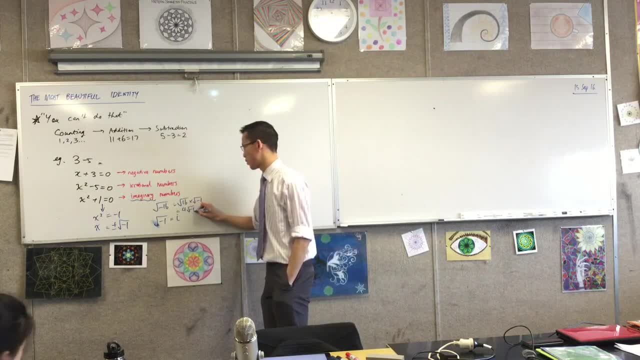 Do you agree, Right? So that's 4 times the square root of negative 1.. So that's 4i. okay, So this is just kind of like your basic building block. You don't need new names for all of these guys. 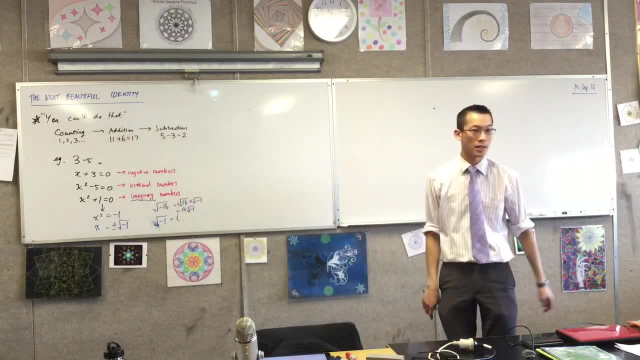 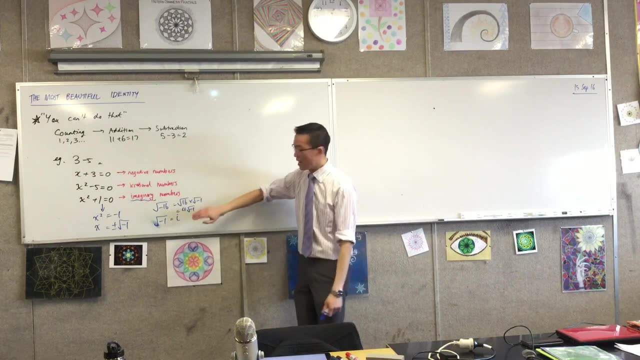 if they're all just bigger and smaller versions of the square root of negative 1, okay, All right. so here's this idea of you can't do that, Well, what if you could? okay, Now we call these guys imaginary numbers. 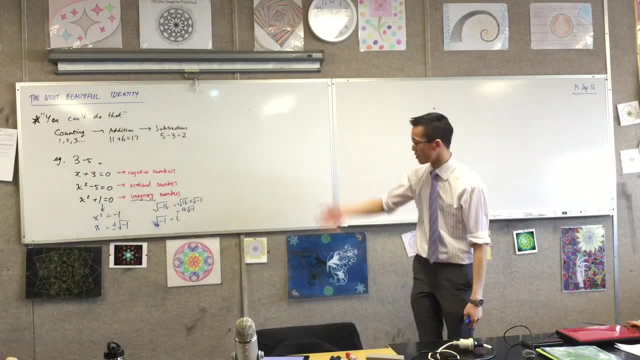 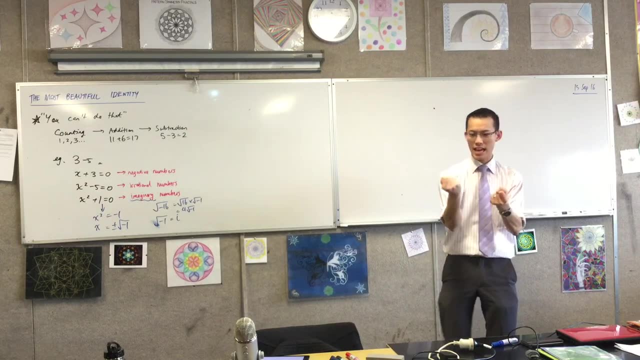 If you put them together with the numbers- you're already familiar with these negative numbers, irrational numbers, et cetera. they're actually kind of like oil and water, right, They don't quite mix together. They stay as the real part, like these guys over here. 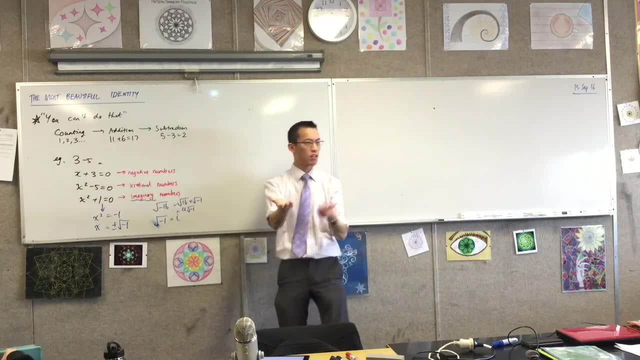 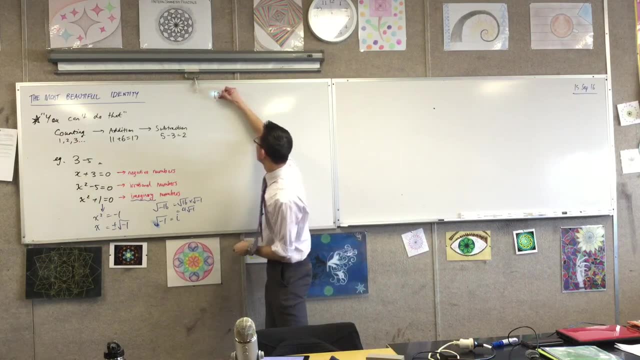 and then there's this imaginary part, which it's almost like algebra. It's like: well, they're not like terms, so you can't just put them together, right, But you can still work with them together, right, Even though, like, say, 2x plus 3y, so it's 7, right?